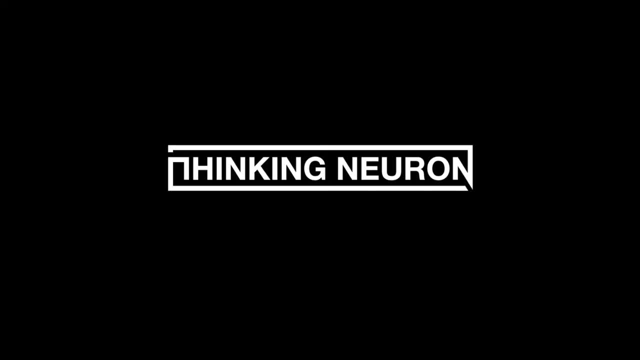 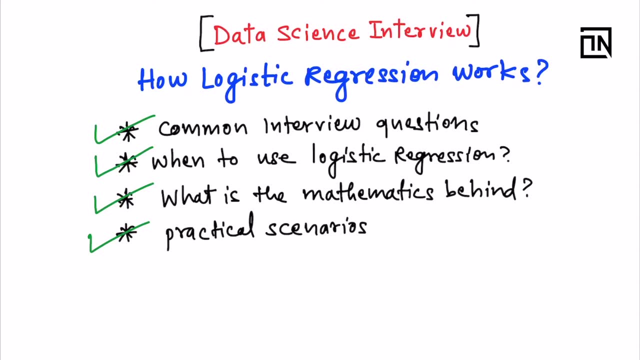 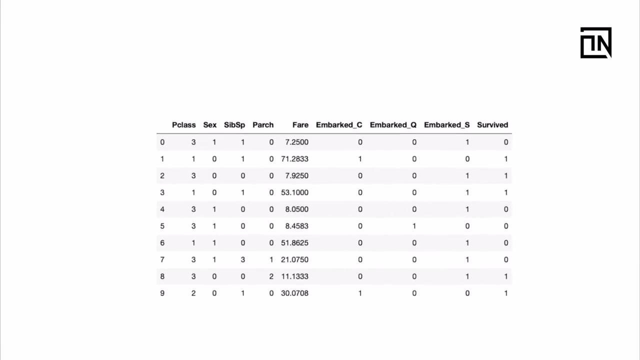 So, as I have discussed in linear regression here also, let me start by a business scenario, which will help you to relate the concept in a better way. So consider this business scenario. and this is a very famous problem: that people who built Titanic. they are now ready with a new version. 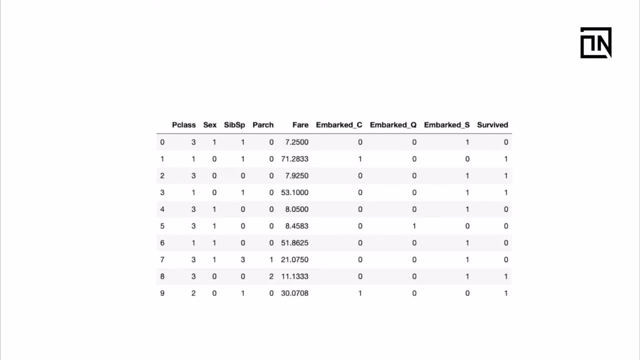 of it. They learned from their mistakes and they now try to build a ship which will not crash given the harsh conditions of the sea. But this time they are also more conscious and they are trying to take advantage of the historical data, The data which 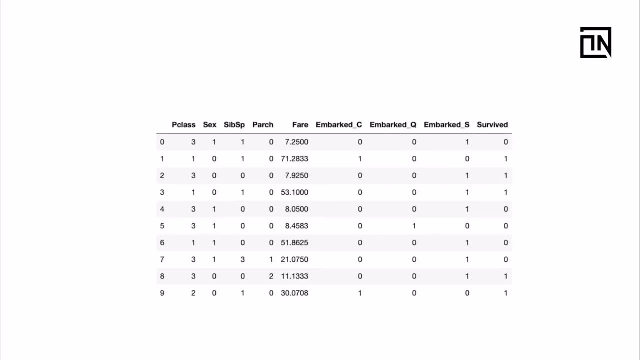 is with them from the previous crash and they want to understand if a person is boarding this new ship and if this ship crashes again, what are the chances whether the person will survive that crash? So they will try to give the tickets to only those people who can survive the crash- okay, being extra conscious. So this is a business. 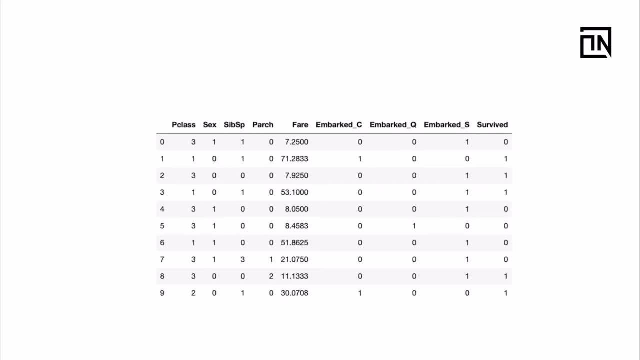 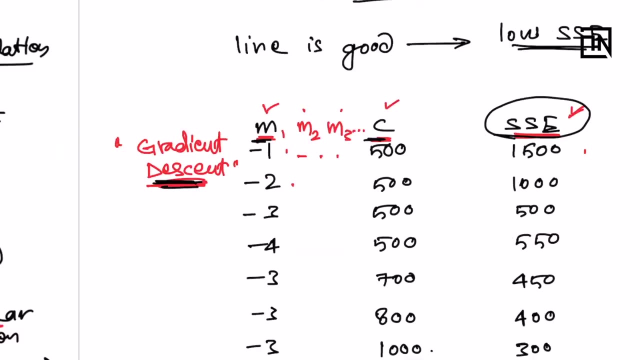 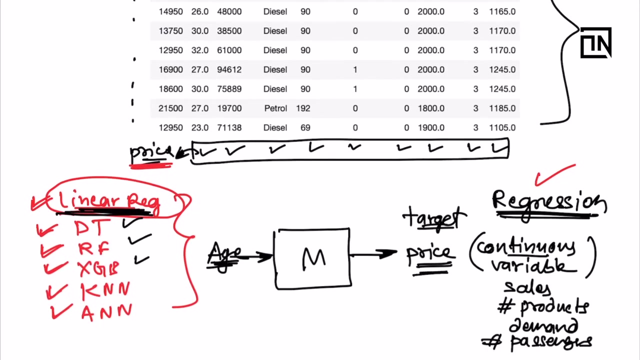 problem, a prediction problem, but as compared to the linear regression problem which we discussed last time, where we were predicting the price of a given car, So we were predicting the price of the given car, So here the target variable was price and the overall problem was a regression problem. 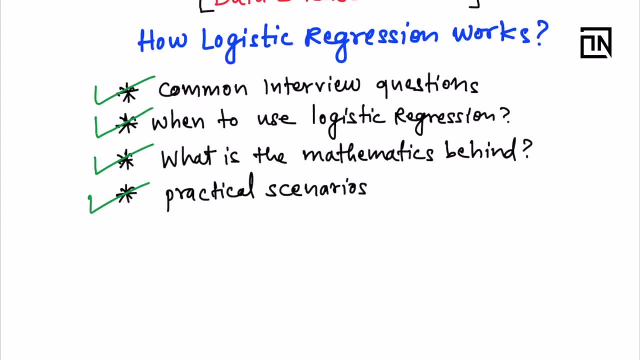 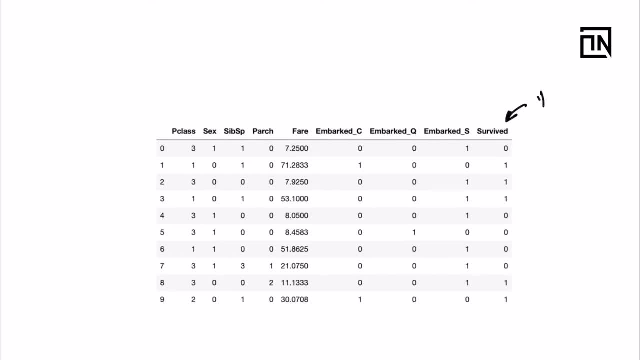 In this scenario? in this scenario, what we are doing is we are trying to predict the survival of a person. this is my target variable and this target variable, even if the values are one and zero, it is numeric, but still what I am doing is classification. So I start with. 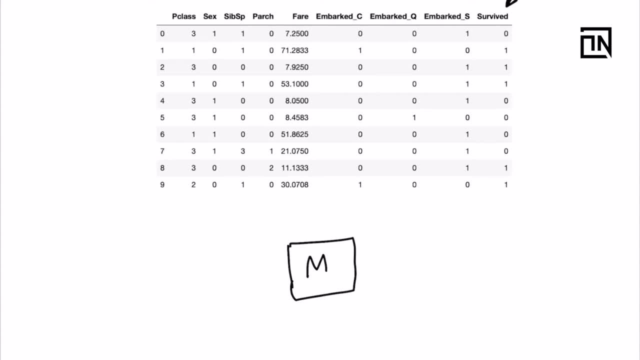 my diagram. as usual, I need to create a model which will predict something. What is that? something? whether a person will survive or not, so the answer is one or zero. the same answer could be in terms of yes or no as well, so these strings can be present, and in that scenario, there is no doubt that this is a 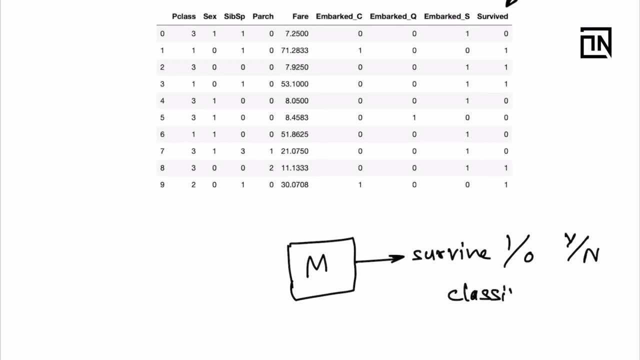 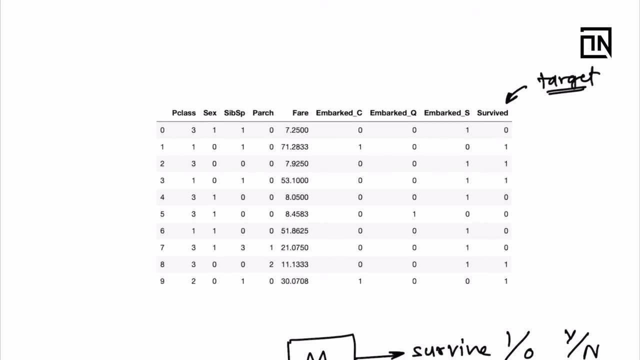 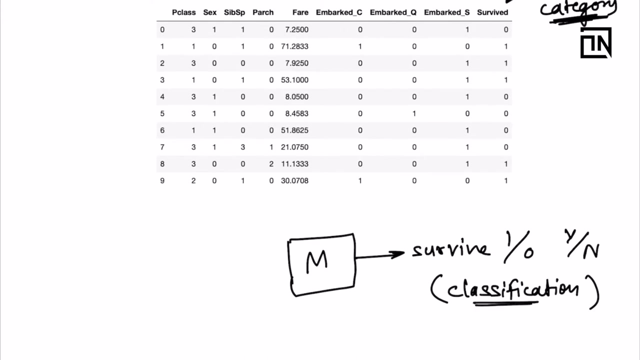 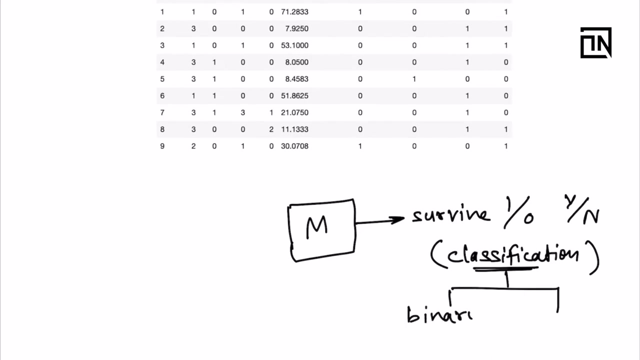 classification problem. when do you do classification? when your target variable is a category, so this target variable, where values are either one or zero, it's a categorical data. whenever your target variable is categorical data, you are doing classification. now, classification can also be of two types. it could be either binary classification or it could be multi-class. 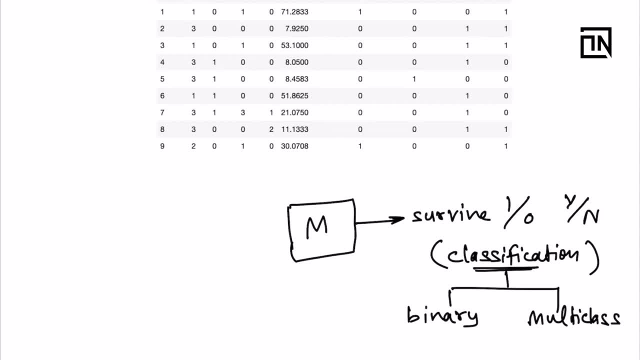 so this is the scenario of binary classification, where there are only two answers possible for the given model, like 1 or 0, or yes or no, or a or b. when there are only two answers, then it is known as binary classification, and this is the case of binary classification. 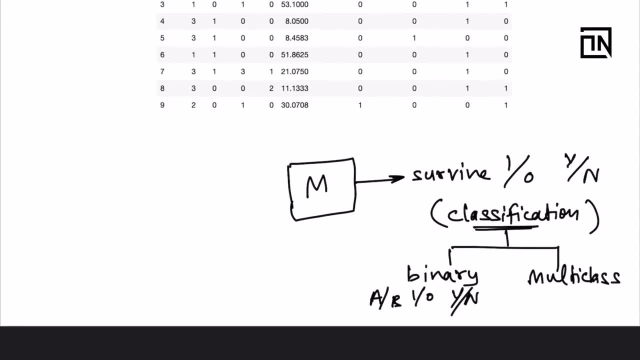 in this scenario, you should use logistic regression whenever you are doing a binary classification in multi-class classification. can i not use logistic regression? you can. however, it is not recommended. so, as a matter of choice, if you have to implement logistic regression, try to do it for binary cases and try to use the other tree-based. 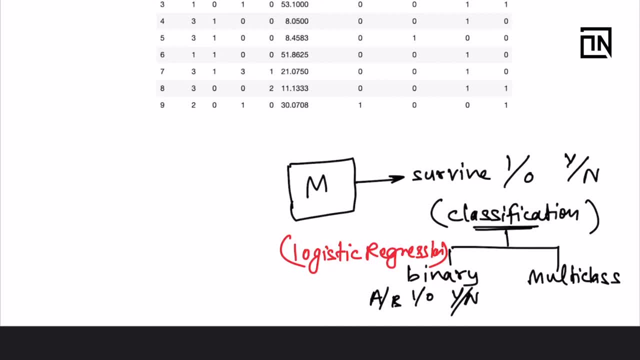 algorithms for multi-class classification, for example, your random regression algorithm, forests or decision trees classifier, or xg boost classifier, or k- nearest neighbor classifier, so on and so forth, or artificial neural networks. so all these algorithms can be used in multi-class classification. so in this scenario, what we are trying to do is we are trying to predict the 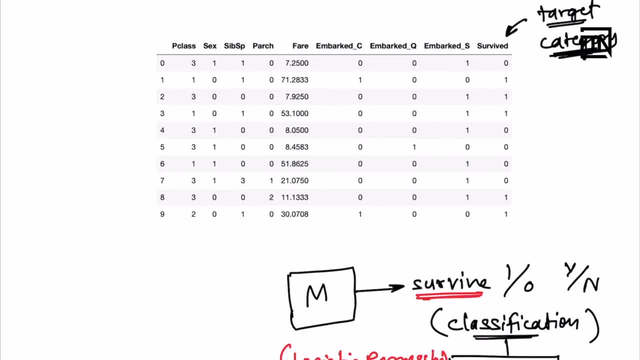 survival of a person, based on multiple factors. so these are my predictors: the passenger class, the gender of the person, the sex column, s i b s p? uh. is the siblings or spouses present on board, the parent or children present or board, how much fare that person has paid and what is the place where the person has embarked the journey or started the. 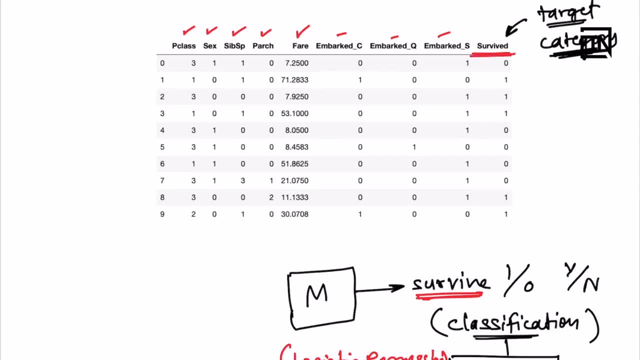 journey and this is the target variable: whether the person has survived the crash or not. so this is the historical data. all this data is given to you from the previous crash. this is historical. okay, from this data, we will try to learn. using these predictors. we will learn the characteristics of a person who will survive the crash, or a person who 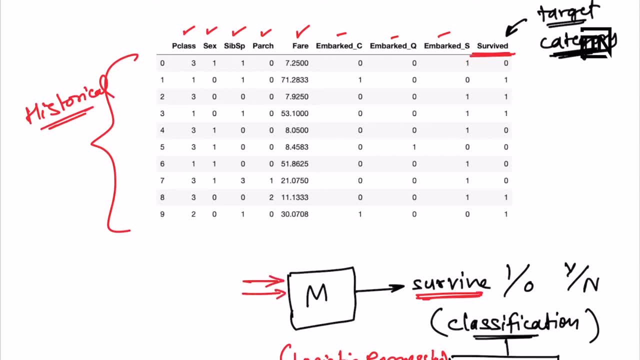 will not survive the crash, right? so these characteristics are what my predictors are. so passenger class, sex column, etc. which of these will be, uh, the final predictors? that is something you decide based on the variable importance charts, so on and so forth. now this data which i am showing you here. i am assuming that you have done all sorts of eda. 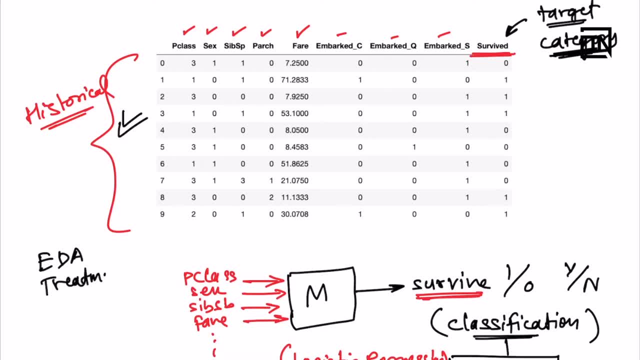 you have done all sorts of data treatment: the outlier treatment, the missing value treatment and the conversion to numeric. everything has happened. and then after that, this data is being used for modeling, and this is the usual way you do all your data pre-processing and then you start with your modeling activity. 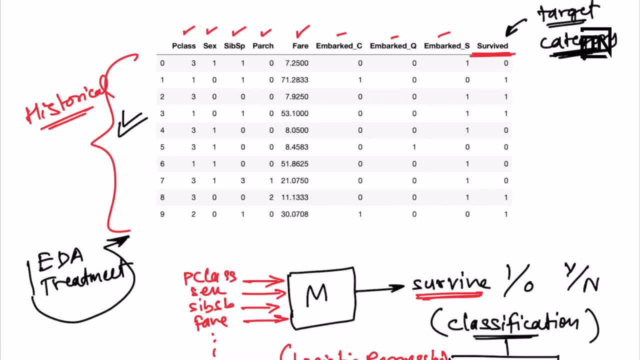 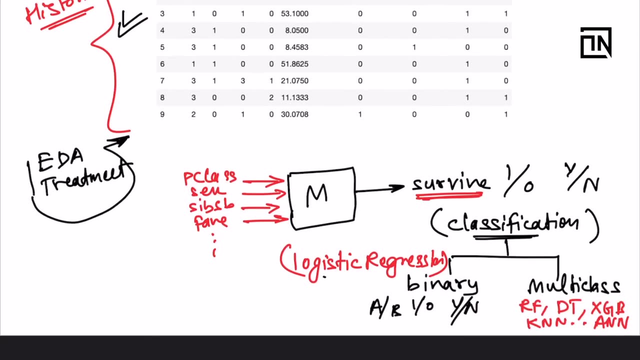 right. so now, out of these, we will try to select some of them now. in this process, we will also learn how logistic regression actually works. we will try to understand what is the mathematics behind it. so now let's understand first of all why this name came into picture: the logistic 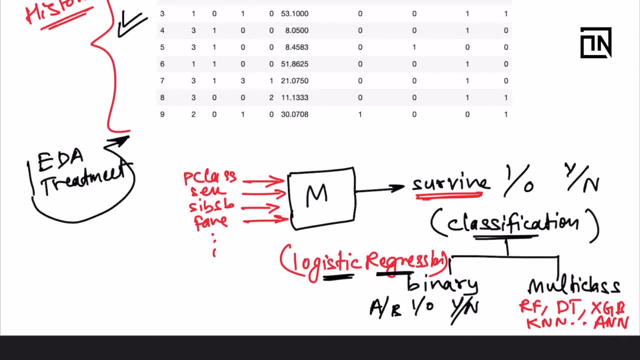 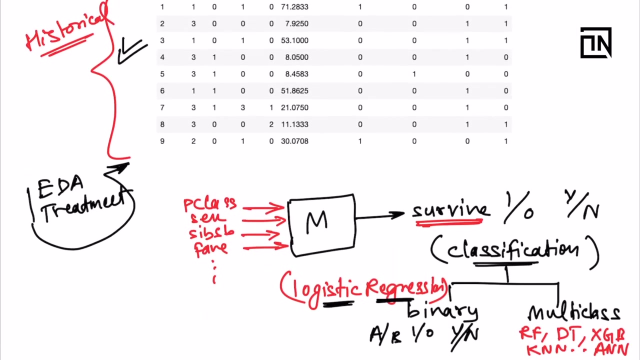 regression, and this is where the theory of logistic regression lies as well. this is sometimes confusing for beginners, because regression is something where you are predicting a number and here we are doing classification. so logistic regression is an algorithm which is used for classification when your target variable is a category. so why, why this name? why regression is present in logistic? 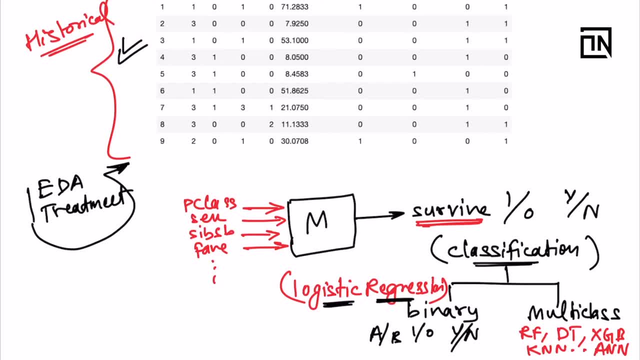 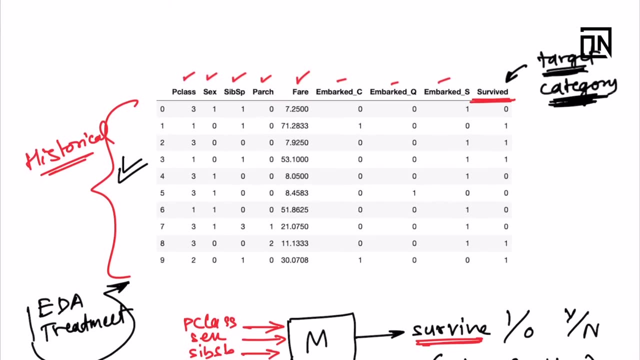 regression because it is derived from linear regression. we did a simple trick to the equation of the line which we had earlier, and we transformed that same equation into a form with which we can now predict classes. okay, so let's try to understand this process. so in your linear regression, things were like this: 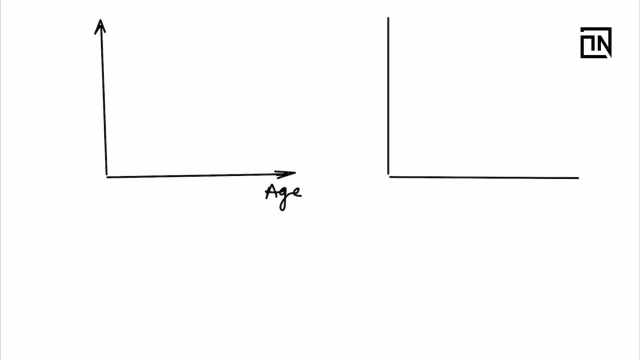 so, if i take the previous example which i gave, the age of the car versus the price, this is what we were predicting. the data was something like this and we created a model which passed through this. so this was my equation of the line and this was my model. using y is equal to mx plus c. i created the equation as price is equal to m times h. 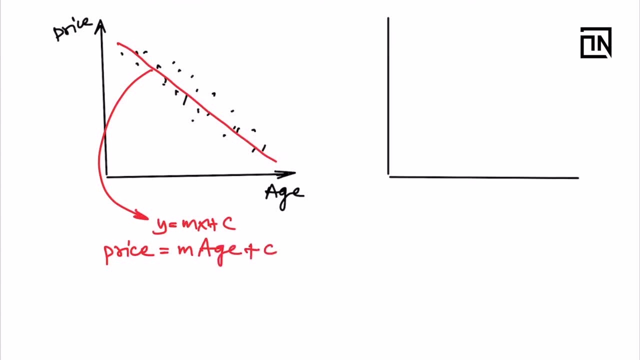 plus c when i did simple linear regression and when i did multiple linear regression. basically, i added more columns to this equation, like price was m1 times h, m2 times kilometer, so on and so forth, plus c. so this was my multiple linear regression and this was my simple linear regression. 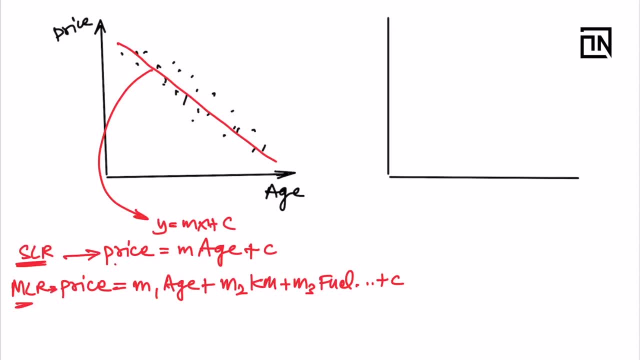 okay, now this equation which we have. this equation is going to give me an output which is a continuous number. all right, that is why we are doing, basically, regression. this is regression scenario. now, the plot which i have created over here. this is also known as scatter chart, this. 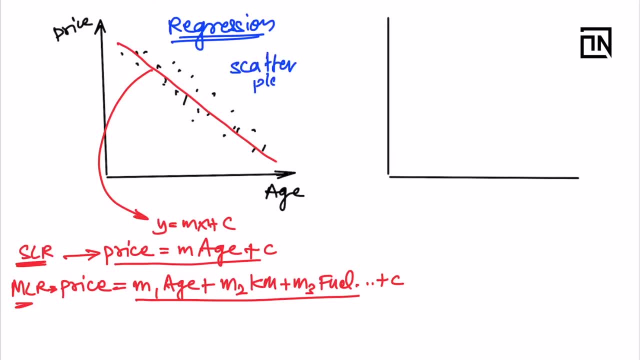 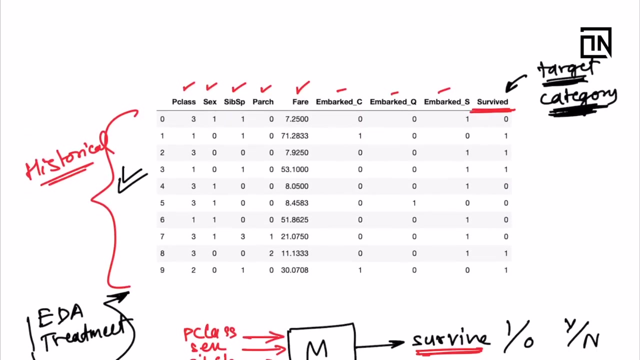 plot is also known as scatter plot. a scatter plot must be generated only between two continuous variables. if both the variables in x-axis as well as in y-axis, if both the variables are continuous, then only you should generate a scatter chart. if you try to generate a scatter chart in this scenario, like consider two: 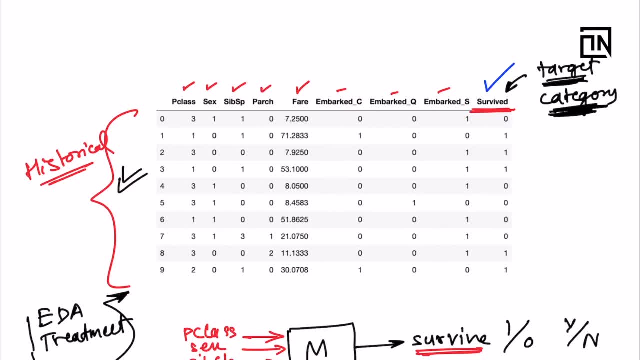 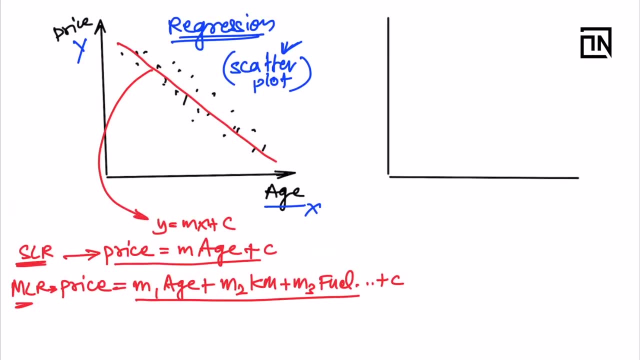 variables. let's say we choose survived and for the, for the sake of illustration, let us try to use fair. okay, so if i draw this over here, in the x-axis i try to draw fair and the y-axis i try to draw whether a person survived or not. it is going to look something like this, because survival is. 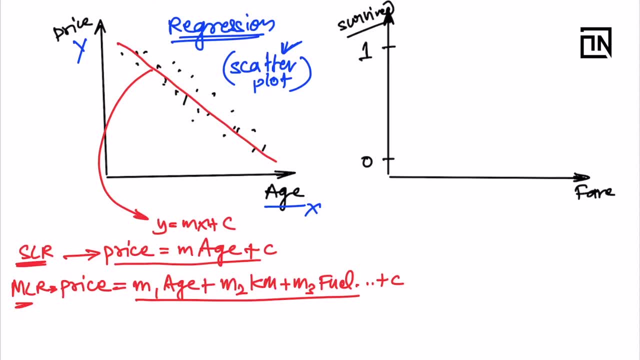 having either value 0 or value 1. so what i will observe is this: these kind of dots will be available. um now, this doesn't really tell me a trend, and this is exactly why we do not use scatter charts between a continuous and a categorical variable. so this is continuous. this variable is continuous. 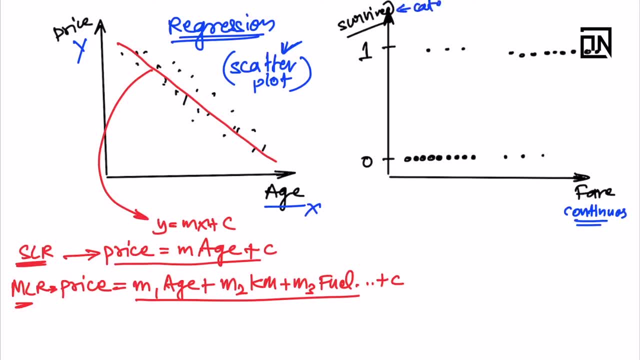 and this one is categorical. the survival- the target variable is categorical. so in these scenarios, what we try to use is a box plot in order to understand the overall trend between the category and the continuous variable, or in order to visualize the relationship between these two variables. 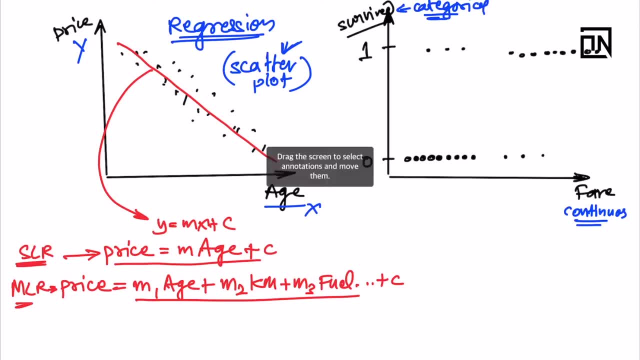 Now, if you try to create the equation in this scenario, let us. let us try to create the equation in this scenario. If I try to write this equation over here between survival and fair, it is going to look like this: survived m times fair plus c, correct? if I try to use the same equation of linear regression, 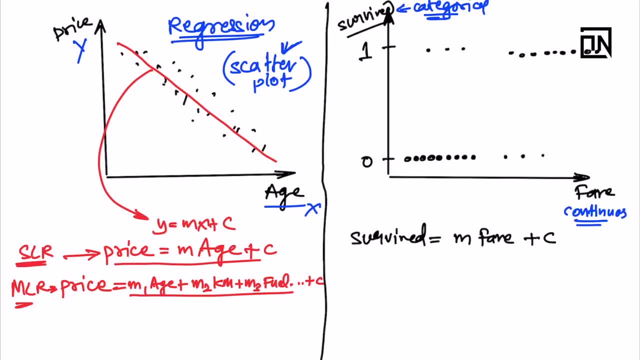 and this will be something like this. the equation will be something like this: This line is not capable of explaining all the points over here. The simple reason is the way the data is present. this particular line will not be able to explain all the data points. 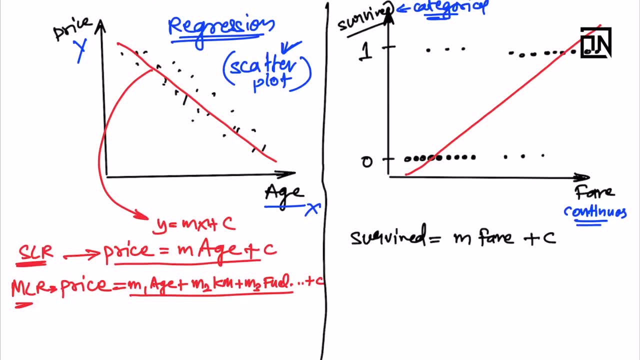 So is there a curve in mathematics which can explain this data? So yes, we have a curve. it's called the sigmoid equation. So the sigmoid equation looks like this now: it will pass through majority of the points, or it will be close to majority of the points. it will miss some of these, but it will be closer to. 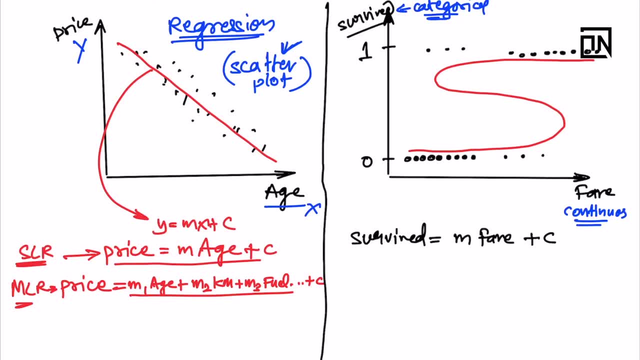 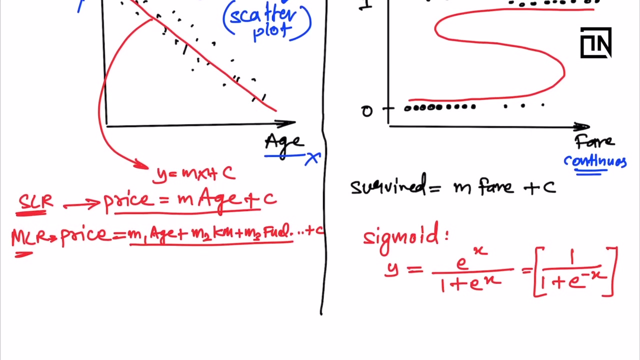 majority of the points. And this equation- sigmoid equation, is known as y is equal to e raised to x, divided by 1 plus e raised to x. or, if you simplify this, 1 divided by 1 plus e raised to minus x. So this is the sigmoid equation, and the beauty of this equation is no matter what value of x you 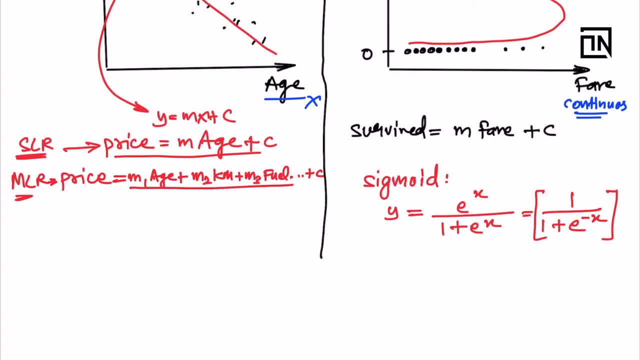 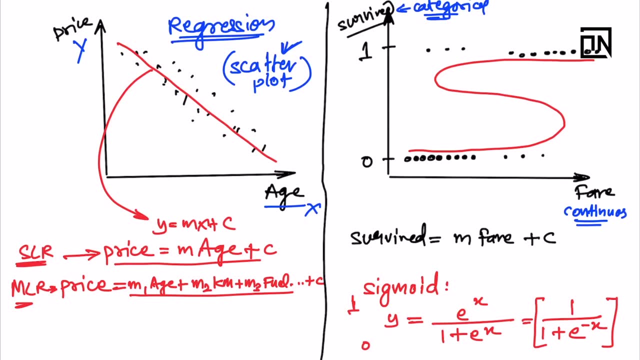 choose you put any value of x in, this output is always going to be between 0 to 1.. It will give certain values based upon whatever input you give, and that value will always range in between 0 to 1, and this is exactly what we want. 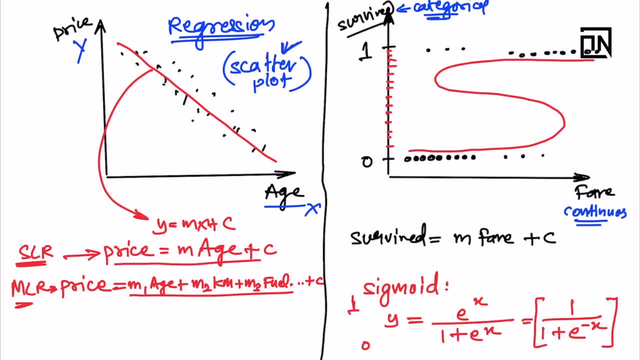 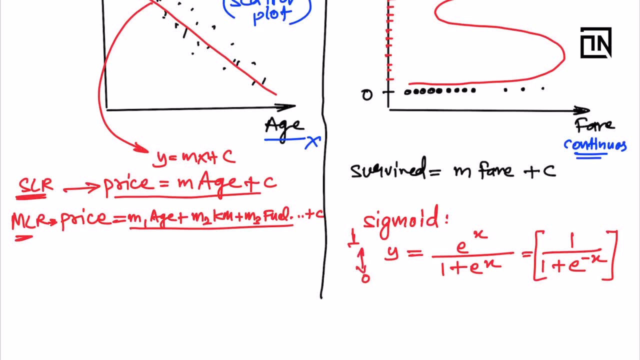 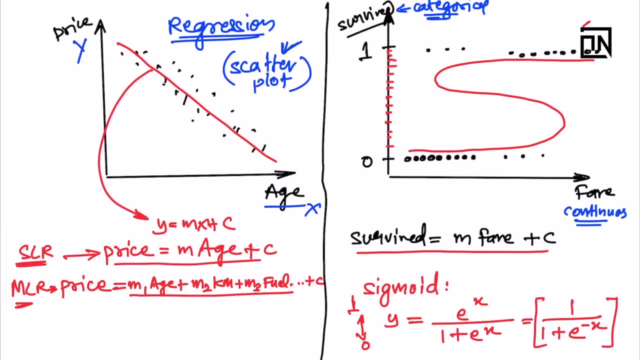 We want the results between 0 to 1, and there is one more thing which varies between 0 to 1. that is known as the probability. So if I can somehow modify this current equation, which gives me a value which is beyond 0 and 1, also like if I do it like this, this can give me for a particular 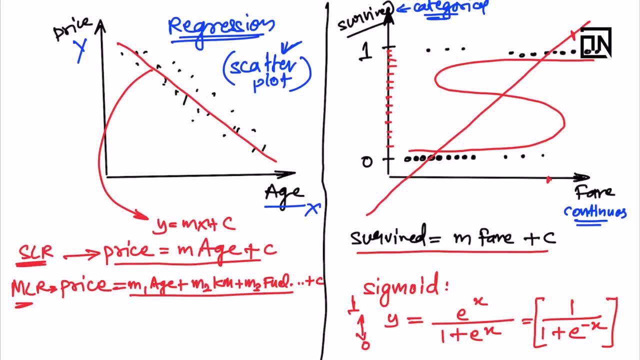 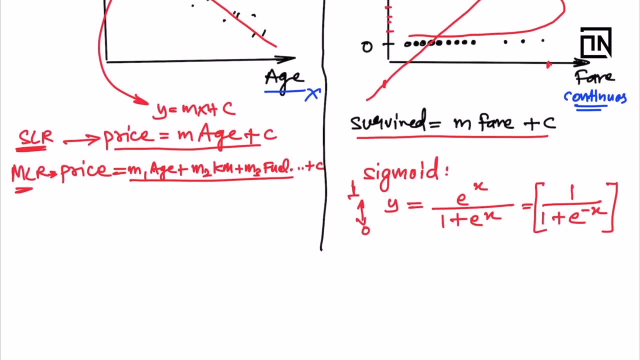 fair. it can give me beyond 1 also. it can give me less than 0 also. values like the equation can give me the linear equation can give me really absurd results. It does not make sense. Sigmoid equation makes perfect sense over here to explain this kind of data. So what I do is: instead of x, I will. 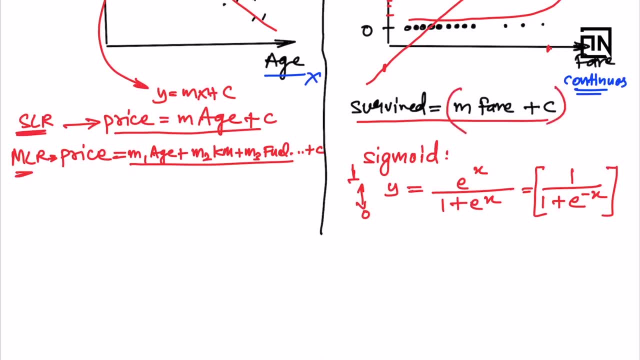 substitute my equation, So what this will become survived is equal to 1 divided by 1 plus e, raised to m, times fair plus c, everything negative. All I have to do now is find the good values of m and c and that will bring out my equation. because this, when I substitute the value of fair for 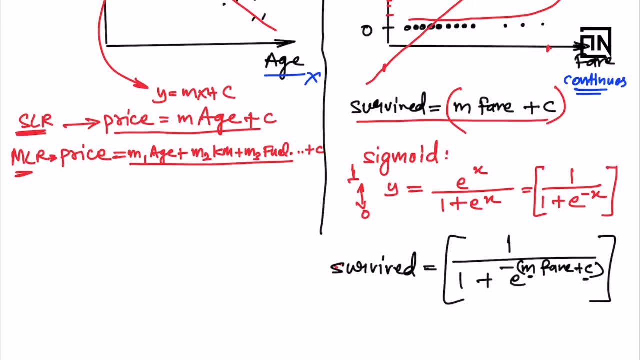 a particular passenger is going to give me a value of survival which varies between 0 to 1.. I can simply say: this is the probability of survival. So what it is going to give me is the probability of survival, which varies between 0 to 1.. 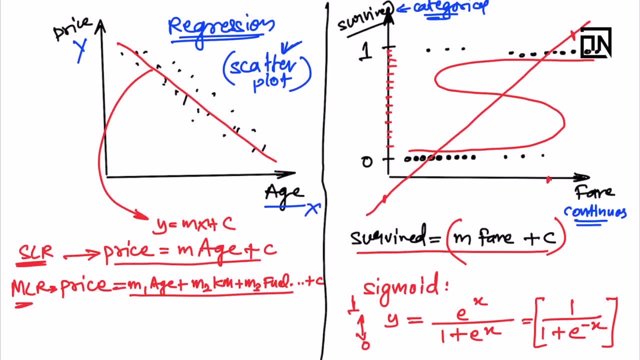 And then I can create a threshold or a rule. I can say that if the probability, let's say, is greater than 0.5, I'll say yes, the person might survive. If the probability is less than 0.5, I can say the person didn't survive. And this makes sense also if you see the data. 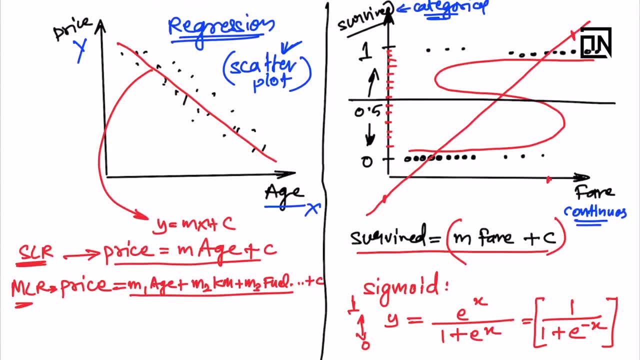 which I have drawn here. let's say, a person has paid less fare, So this person is probably traveling in the third class and the chances of that person's survival will be less. Some exceptions might be there, okay- who have paid less fare and still survive, like these. 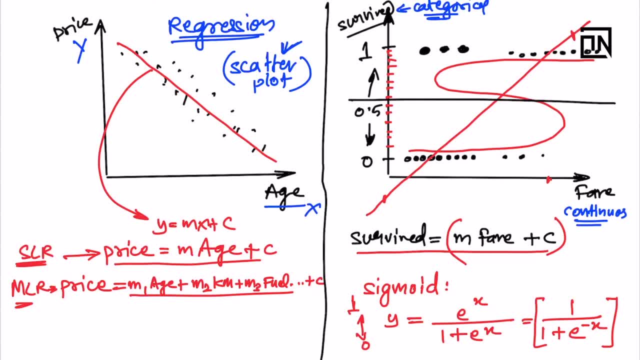 But many people, or majority of the people, will die. Similarly, if you have paid high fares, most of the high fare people will survive And there might be some exceptions who have paid high fare but still did not survive. So it makes sense that the probability which will be thrown to me 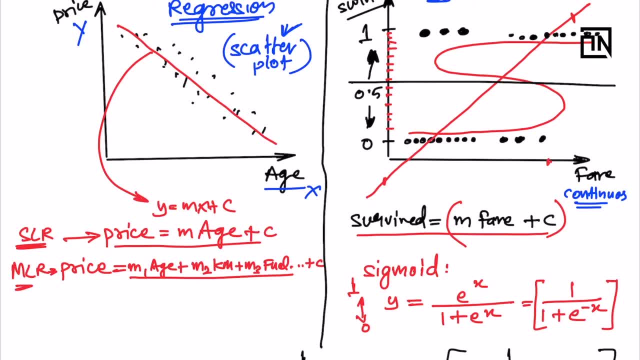 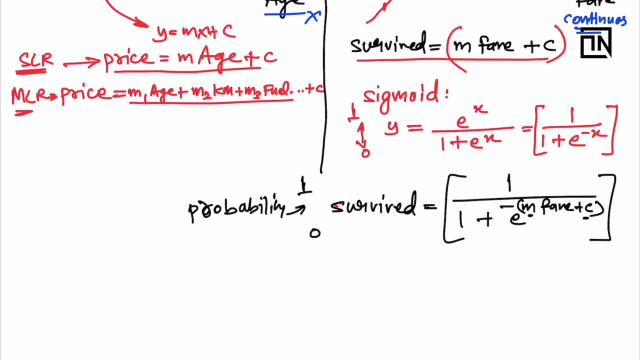 by this equation will describe this extent. If it is greater than 0.5, I will say, yes, the person will survive. If it is less than 0.5, I will say the person will not survive or the chances of that person's survival is very less All right. so this becomes my equation. 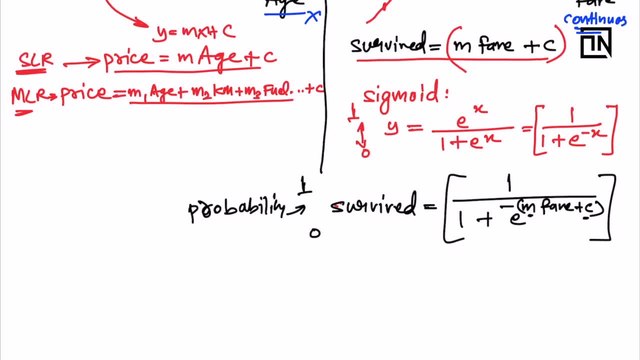 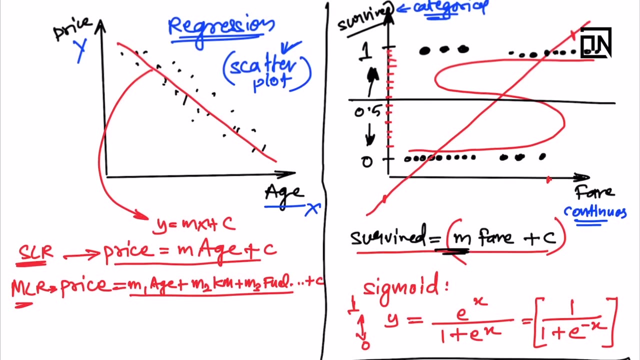 And if you simplify this, this is nothing but your logistic regression equation. So this is where this name regression came into picture, because it is derived from the linear regression equation by taking it to the top of the sigmoid function, which is able to explain this kind of 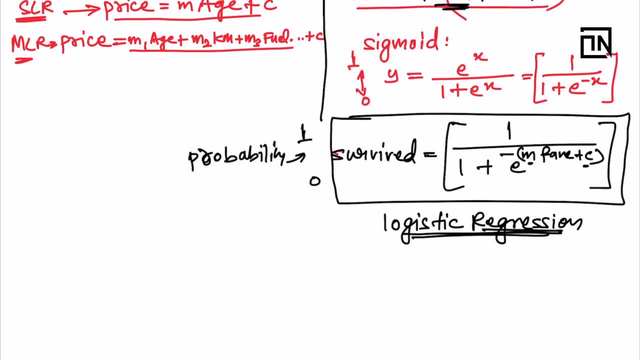 data- Okay, and this logic function is created. So my equation of logistic regression is this: Okay, what I'll get from the logistic regression equation is the probability of survival- Okay, and based on that I can do my predictions whether the person will really survive or. 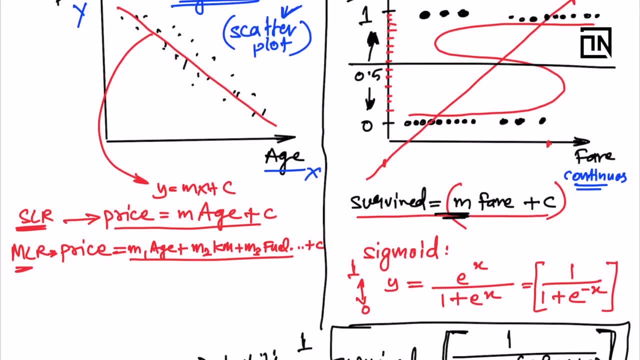 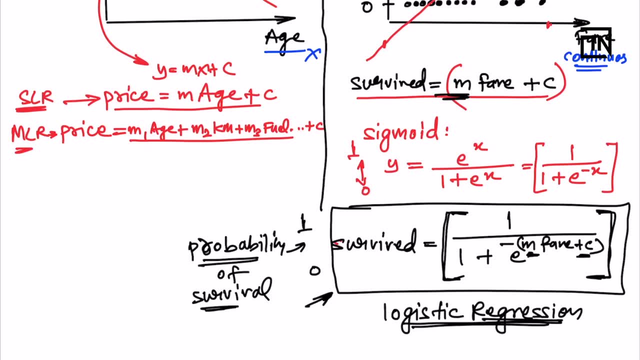 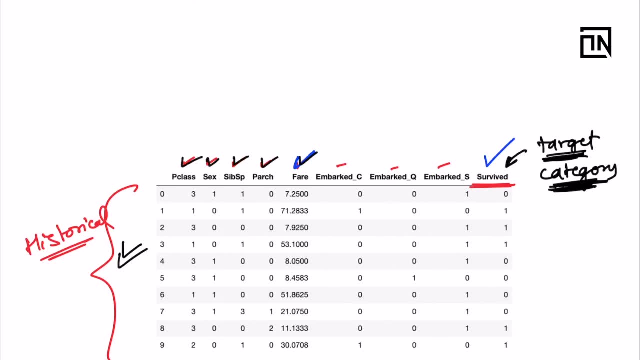 won't survive. Now, just like linear regression, we have to find the values of m and c over here And if there are multiple predictors which we are using, like after fare. we have used parent, children or SIBSP or sex or passenger class. 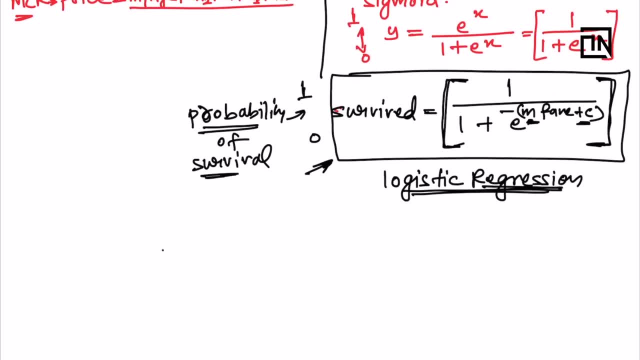 how my logistic regression will look like. it will look like this. So there's some other attributes there, right? So I will give you a little bit about it. So I'll go to the next slide here, And these are my other options here. 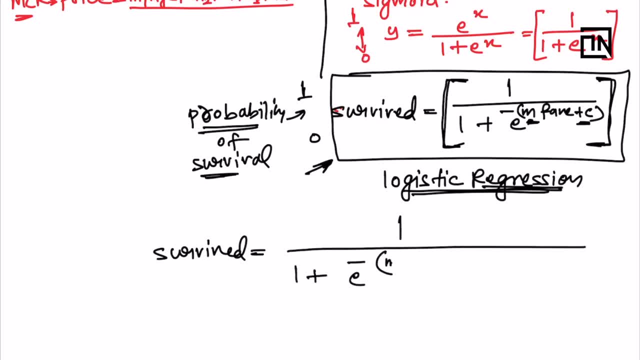 So here we'll go to this column and I'll do this column. So let's go to column e: raise to minus m one times fare plus m, two times parent children plus m, three times column, and so forth plus C, So all the variables which you have chosen. finally they will go here and all I have to. 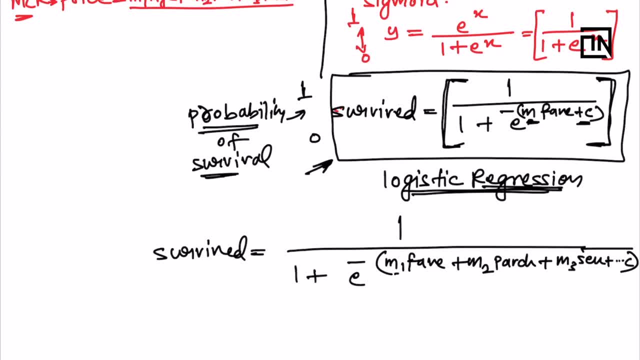 do is find out the values of m one and two and three, etc. So if you have not got the values that you want, you can just scroll down, And if you have not got the values that you want, you can go here And you can see that if I have not got the values that you want, I'll be able to find them. 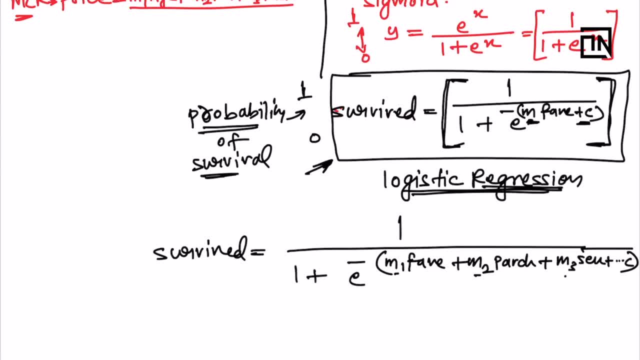 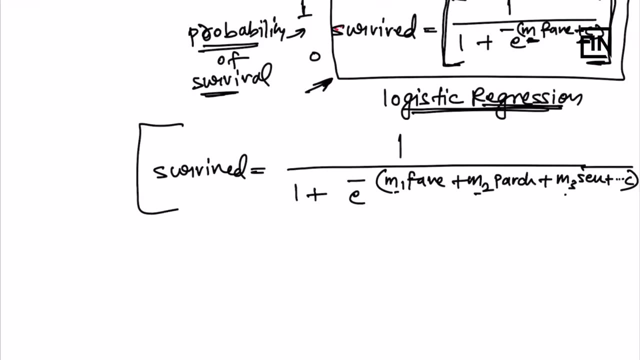 have not seen the linear regression video. i'll highly recommend that so that you understand the process of the gradient descent which happens and the way we find the values of m1, m2, f3, etc. all right, so this becomes your final equation for linear logistic regression. so in linear regression, 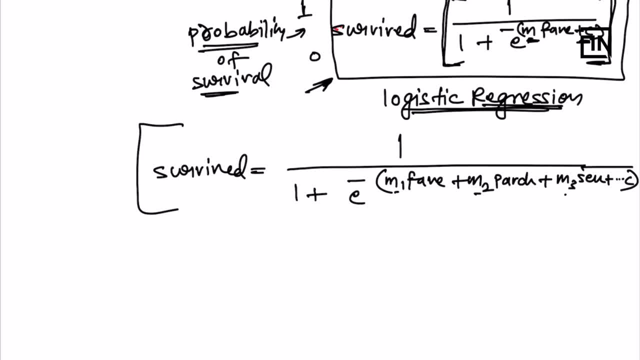 we had the sum of squared errors which we found, and we tried to reduce it. that was our cost function. here, our cost function will be something else. it is known as the maximum likelihood estimation process, and what we estimate over here is the maximum likelihood of these coefficients. 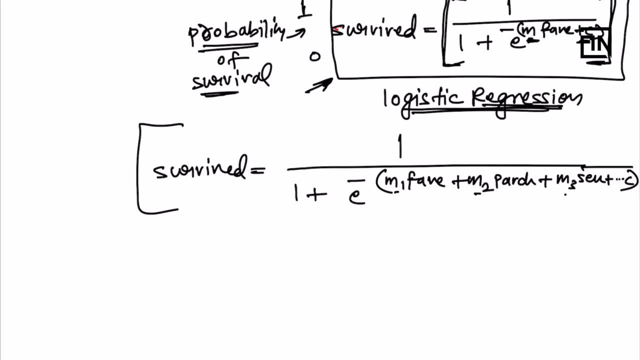 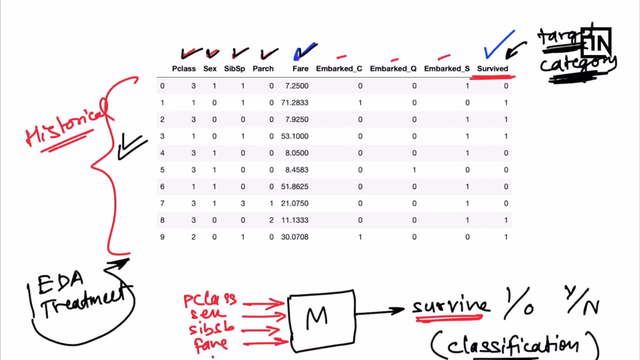 being the best coefficients. so this is all sounding really complex, so let us try to break this down into set of simpler steps. so in this data, if you see, the survived variable is my target and what i'm predicting is the probability of survival right. so let's let's try to redraw this and understand how logistic regression works. 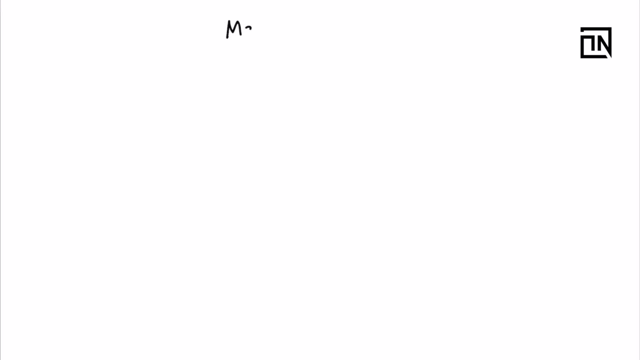 internally. the process is known as maximum likelihood estimation. so how do we build this? so you have your data and you have. you have your target variable survived. what you are predicting is the probability of survival, the probability of survival. so if the original value was 1 0 0 0, 1 0 0, something like this: 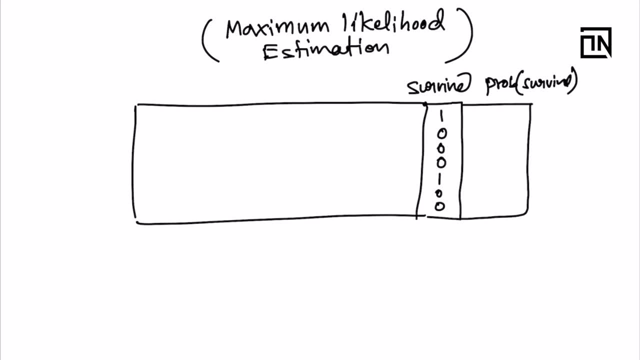 so what you want from your logistic regression equation, this equation, what you want as an output from this equation, is, if the actual value is 1, the probability which this equation should give you should be higher. higher than what? higher than, let's say, 0.5. so some somewhere between, let's say, 0.8 and. 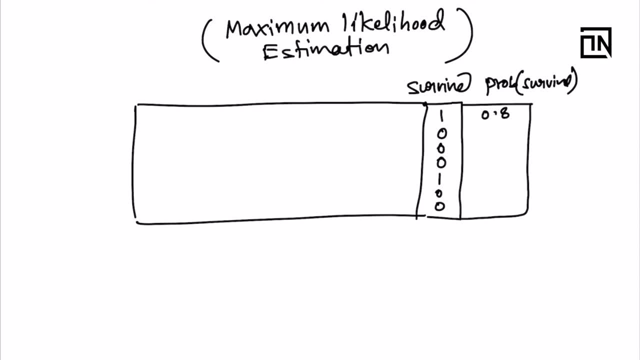 if the survival value is 0.. actually, the person did not survive, so the equation which you are going to build should give you a result which is low, lower than 0.5 specifically, so let's say 0.2, 0.3 or 0.4. 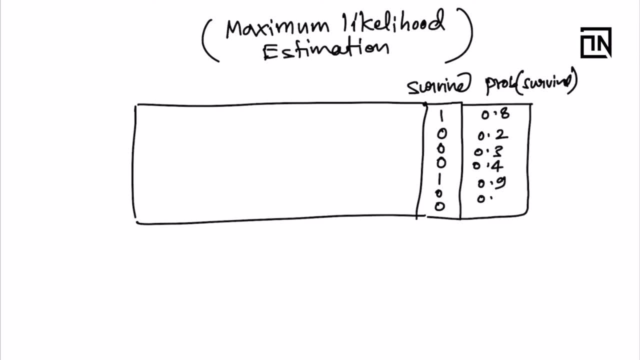 and here let's say you're got 0.9, 0.2, 0.1. so, as a final prediction, what i can say as a final prediction, as a final prediction, i can say: the probability of the survival is 0.8 means it's very high. 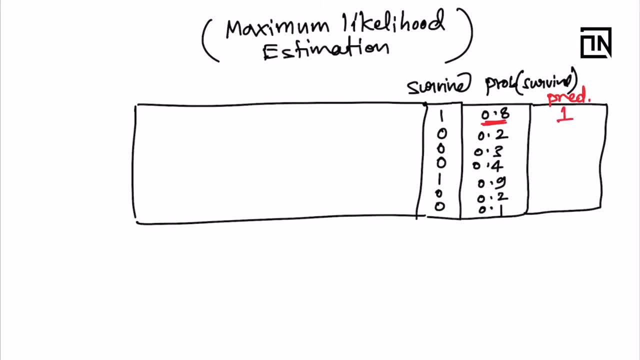 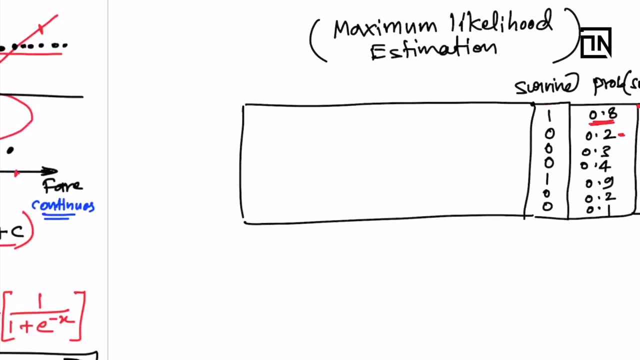 probability, my answer should be 1. if the probability of survival is 0.2- so the person will not survive- my answer should be 0, so on and so forth. so, based on the probability, i am able to do the prediction by using this threshold and that creates the prediction. 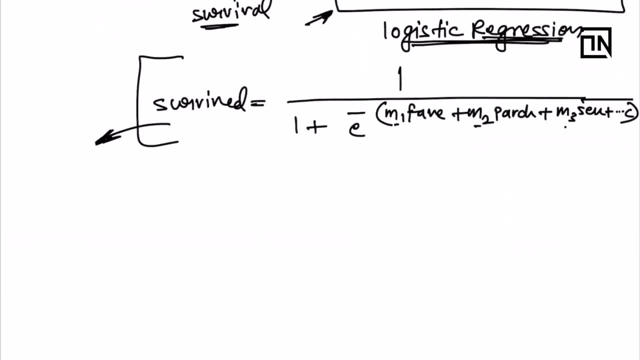 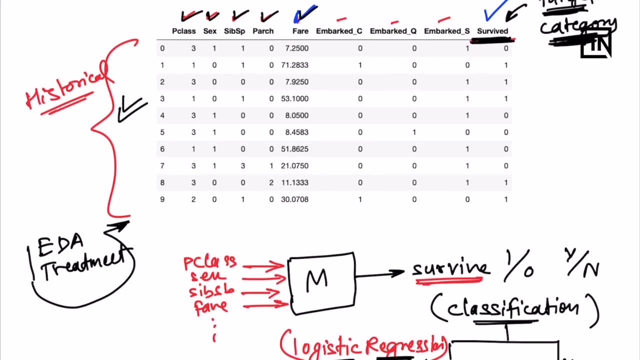 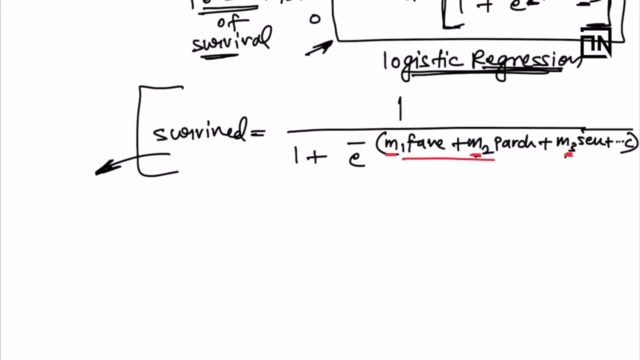 column. so i need to find out such kind of values of m1, m2, m3, etc. so that for every row of data when i input passenger class x, si, b, a, i, next SP, Parge, fair all these values in my equation. which equation? this equation, when I feed all 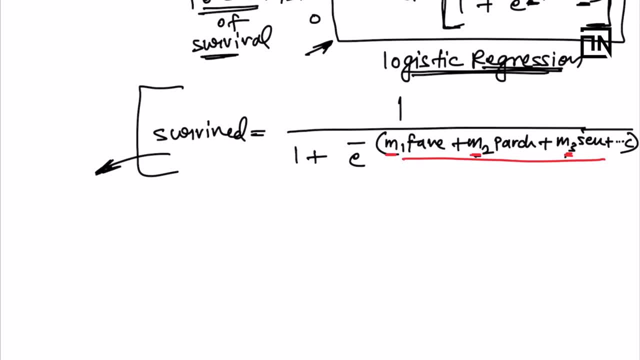 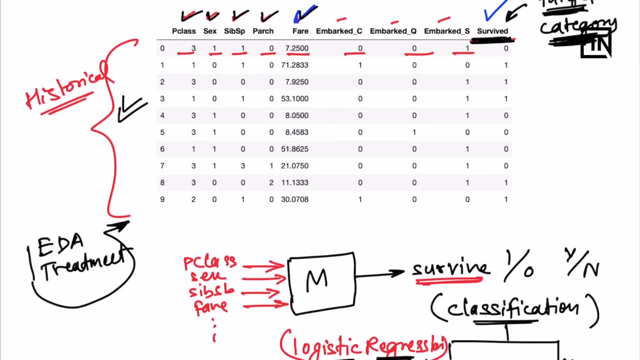 those values. so these m1, m2, m3 should be such that the result which is coming over here, which is between 0 to 1, it should come close to the actual value which was there in my training data. so if it was 0, the probability should come close to 0. if it is 1, then the probability should come. 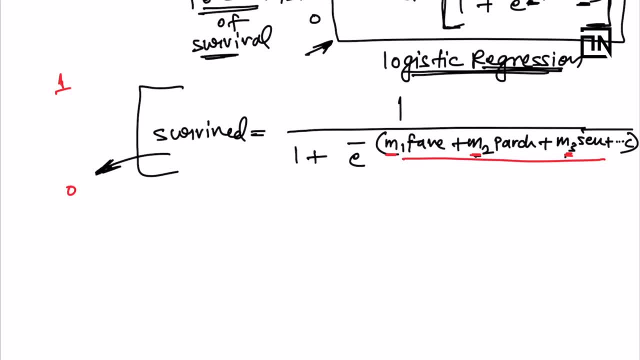 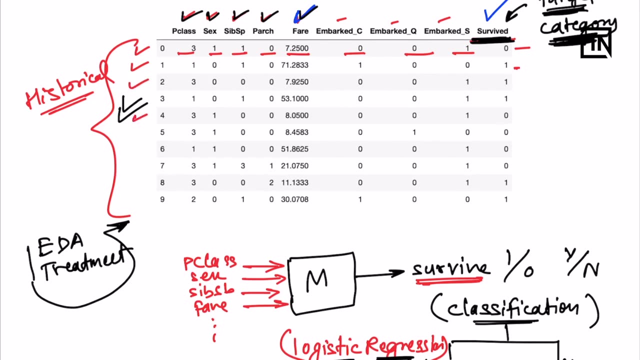 close to 1 right, so that that way I'm able to explain the training data which I have and learn the patterns properly, because I have found out such values of m1, m2, m3, which are explaining all these data points. okay, so this is what is done as an iteration based on the maximization of the 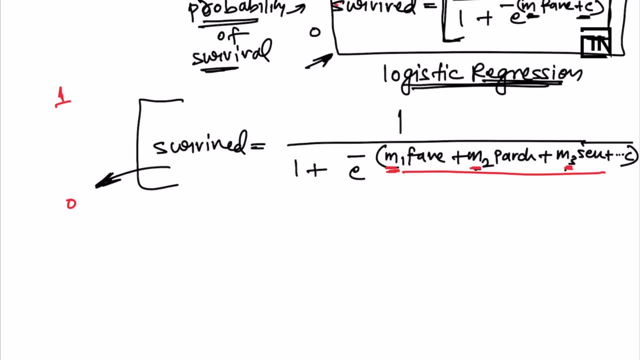 probability. so what we are maximizing here? the probability of survival given a particular row of data. we are maximizing the probability of survival given a particular row of data. we are maximizing the probability of survival given a particular row of data. we are maximizing the probability of survival given a particular row. 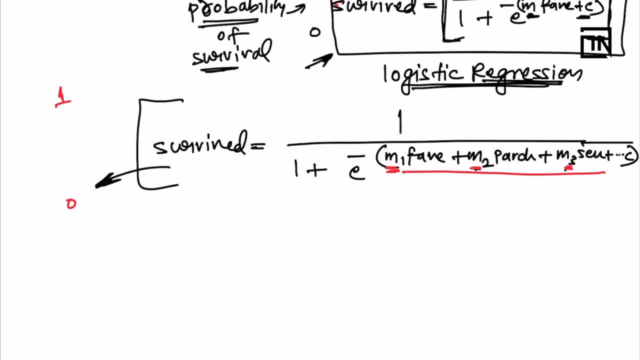 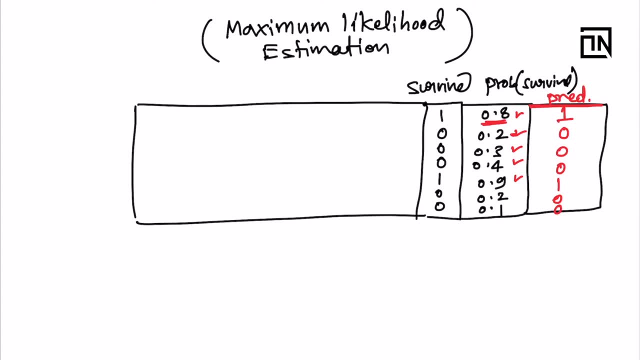 of 1 as close to 1 and 0 as close to 0. okay, so I expect my model to give me these kind of results and accordingly, I'll do the predictions. so what are these kind of values of m1, m2, m3 and C, which? 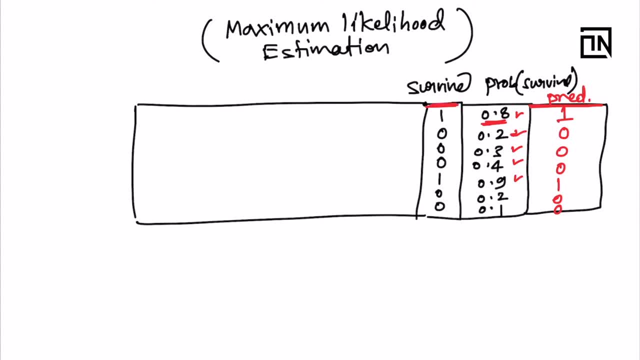 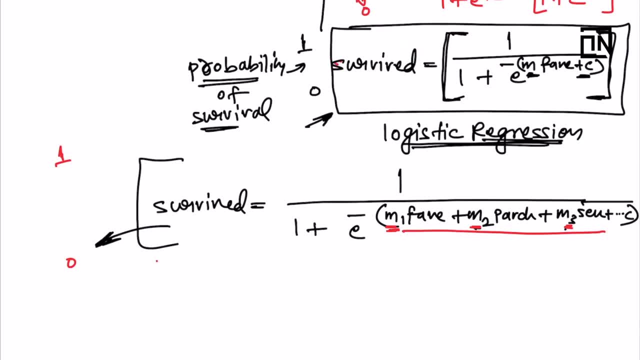 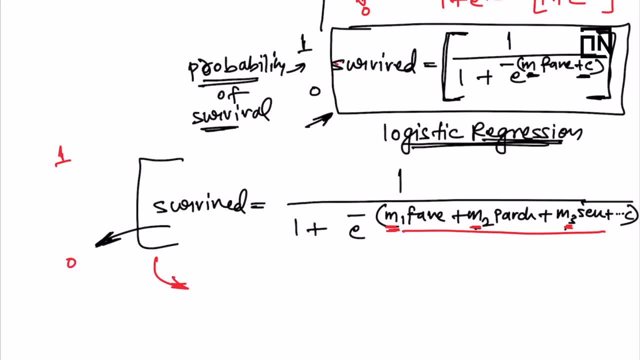 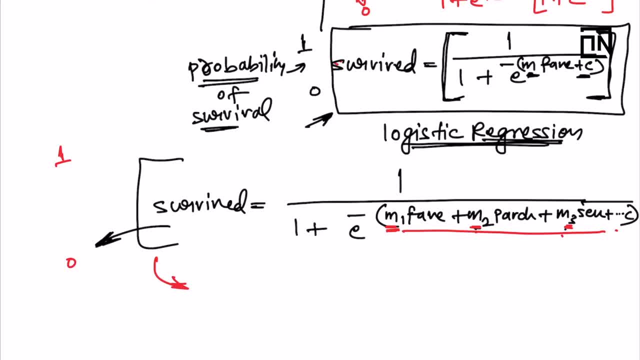 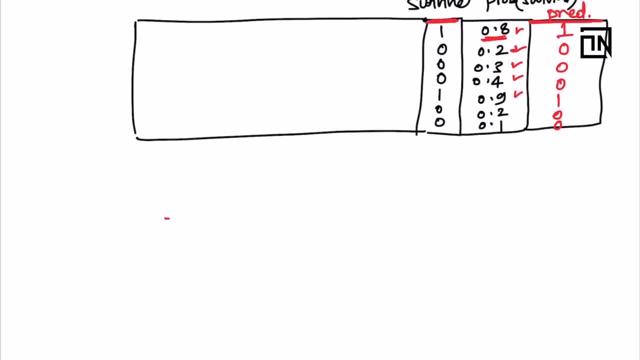 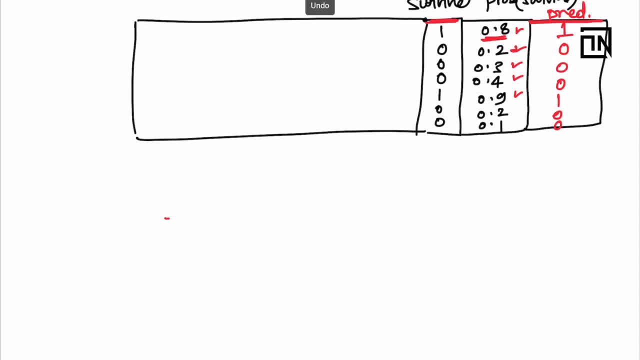 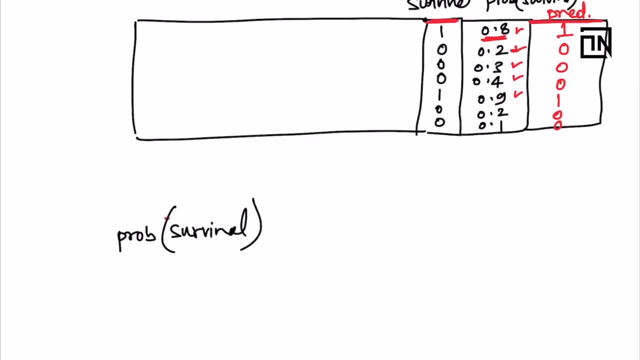 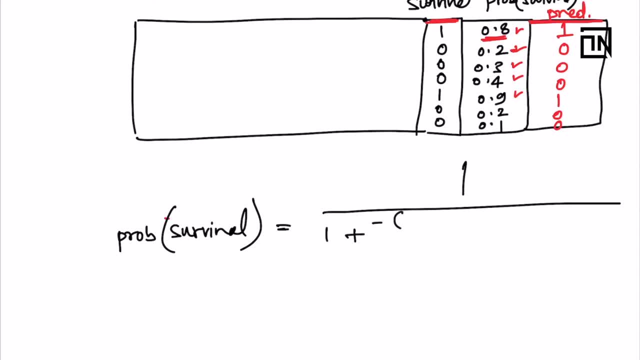 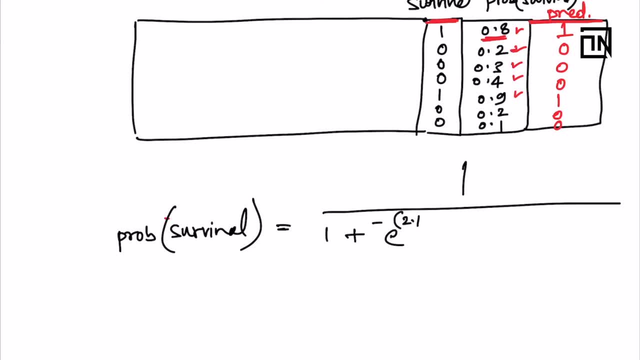 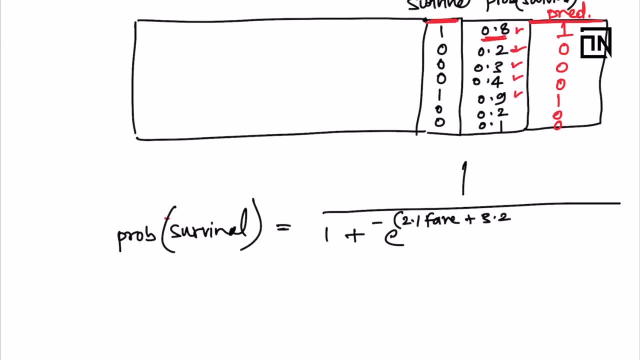 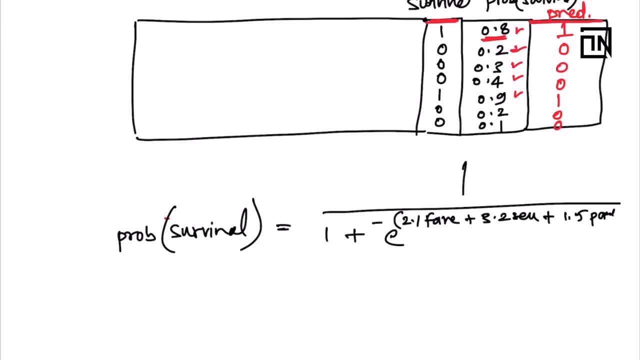 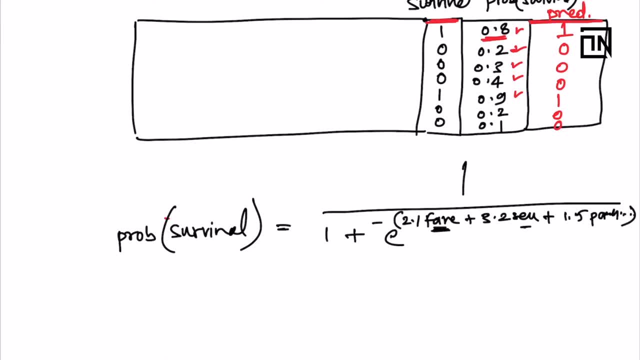 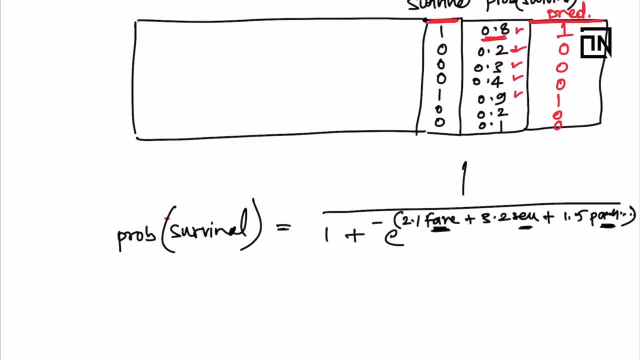 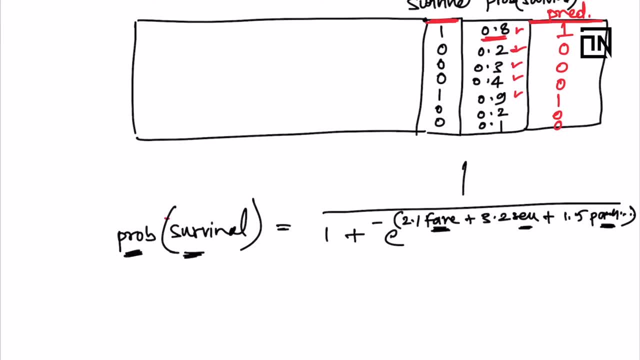 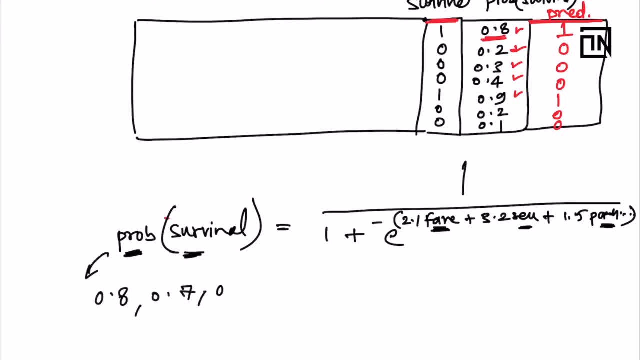 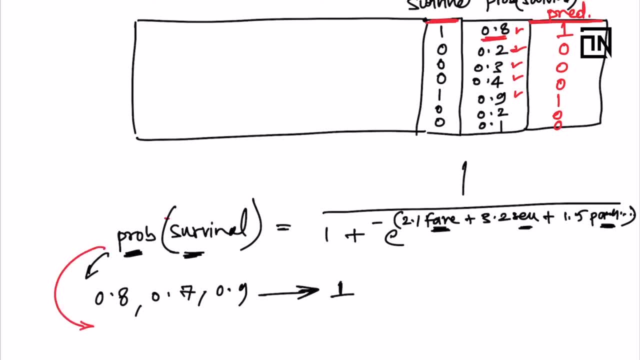 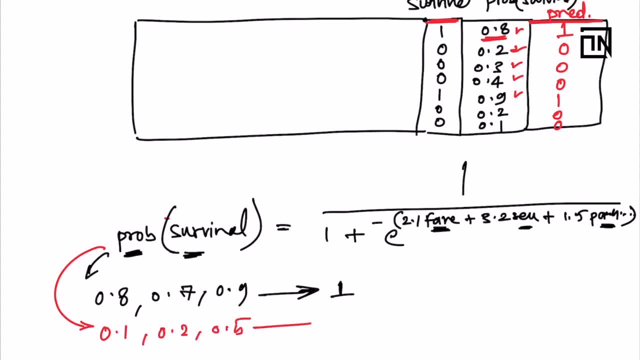 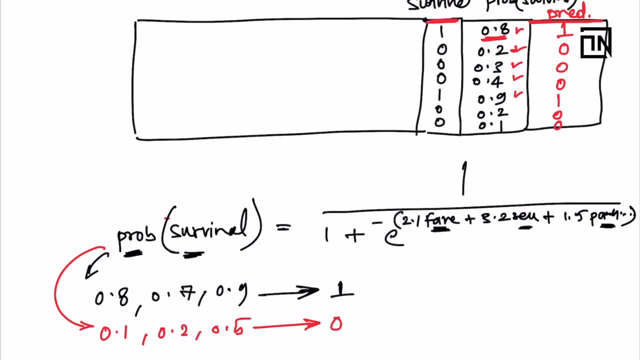 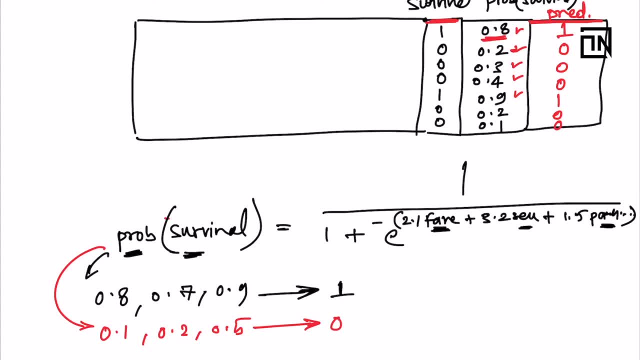 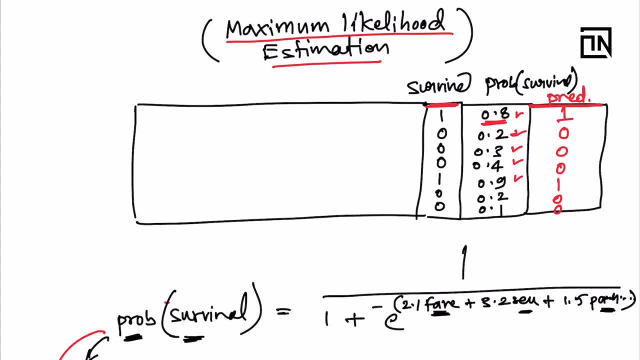 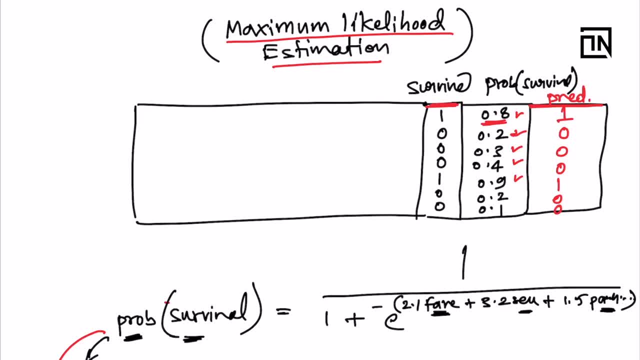 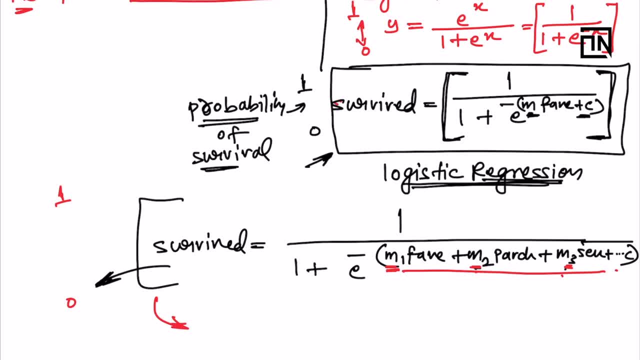 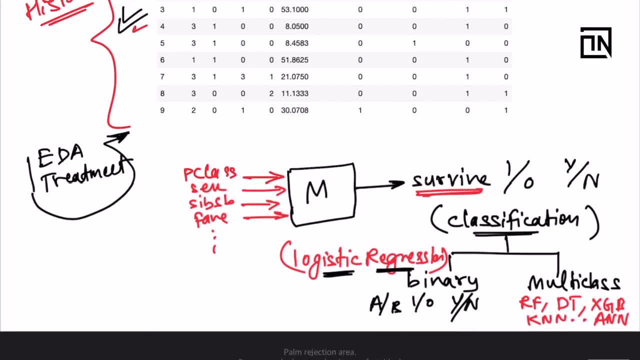 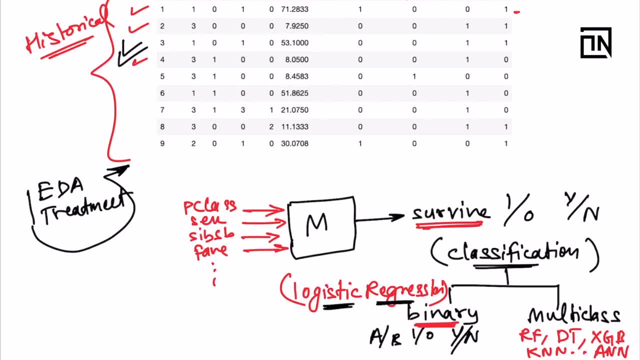 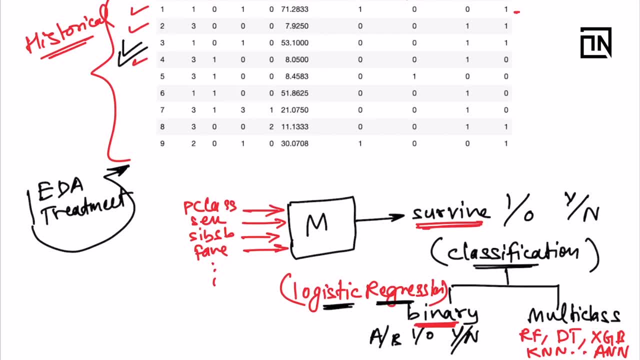 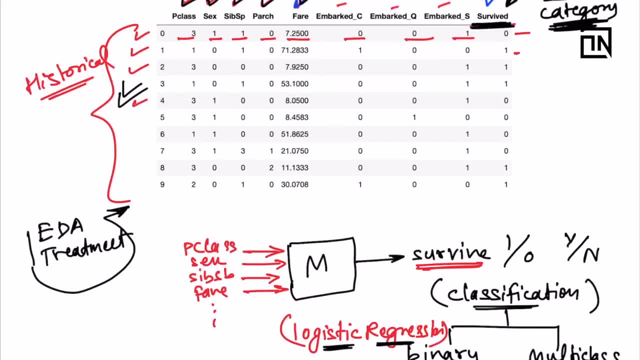 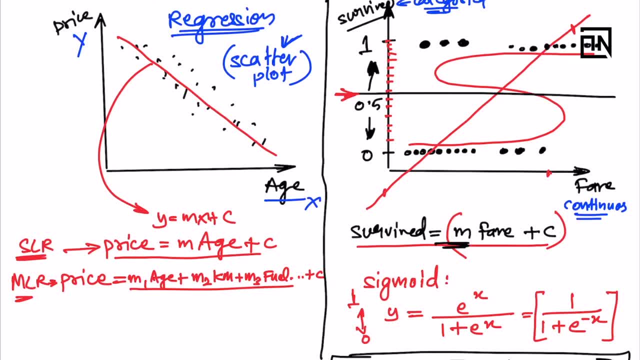 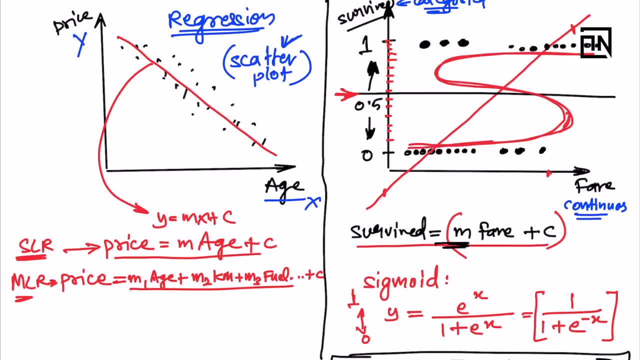 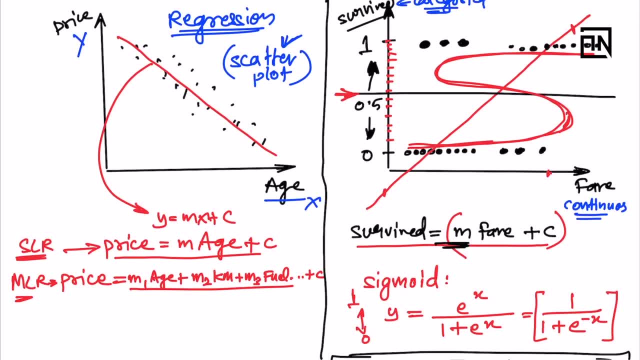 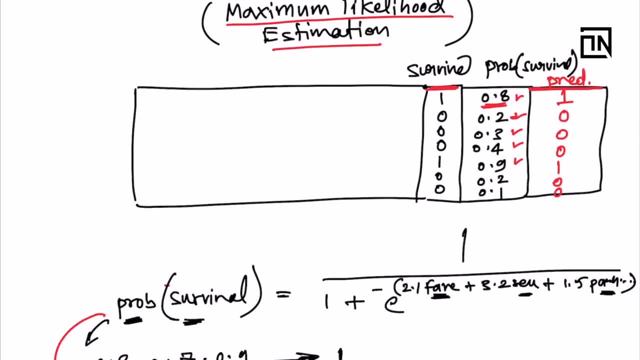 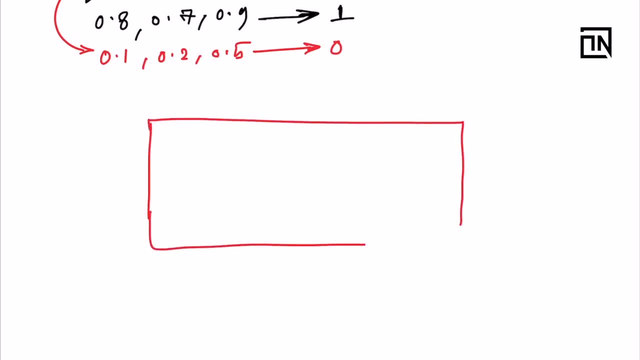 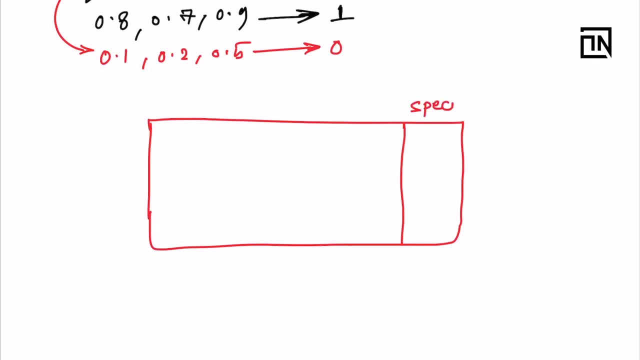 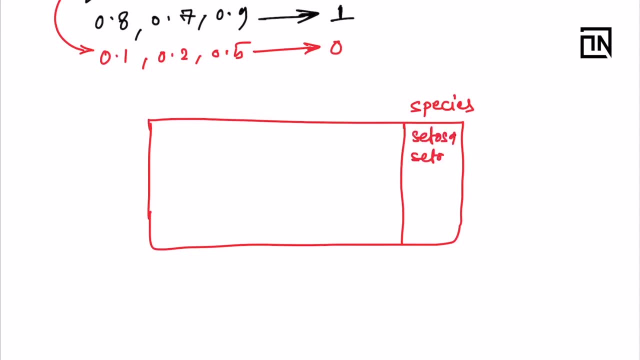 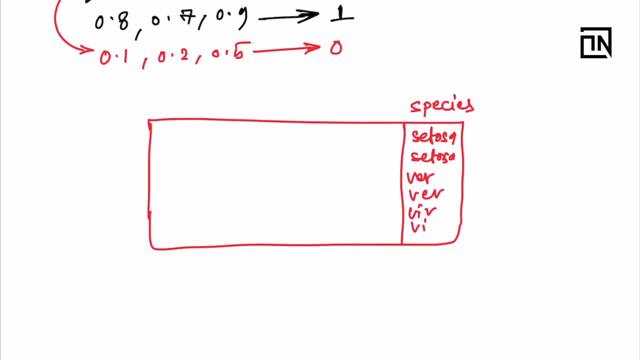 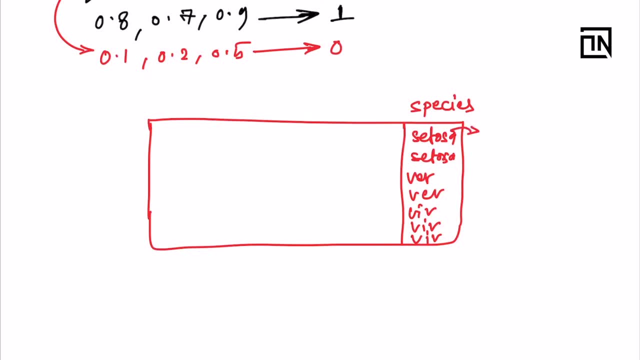 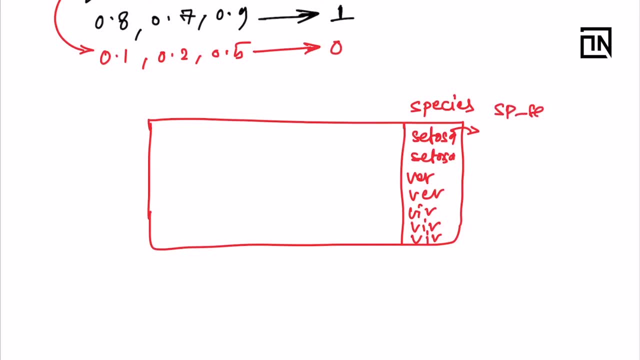 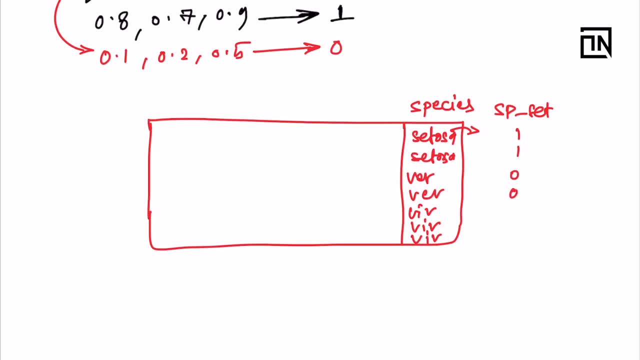 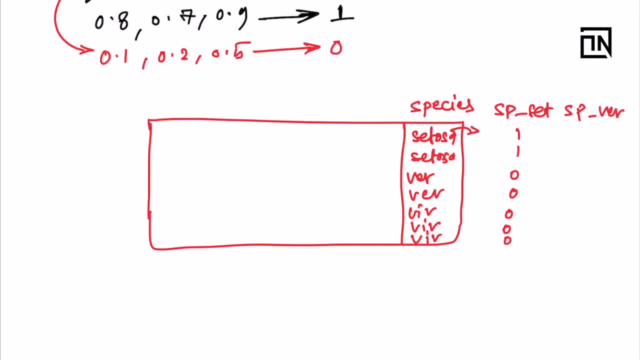 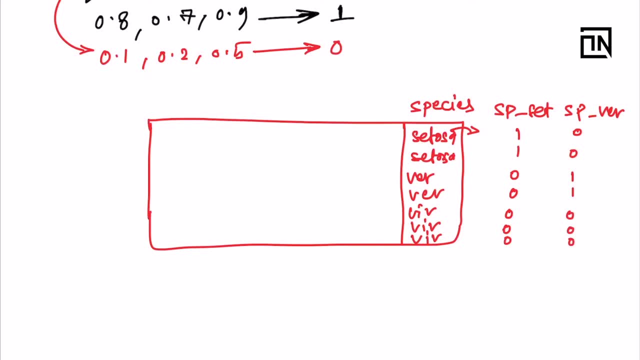 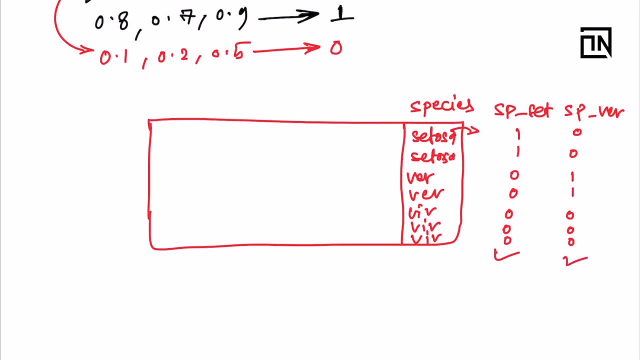 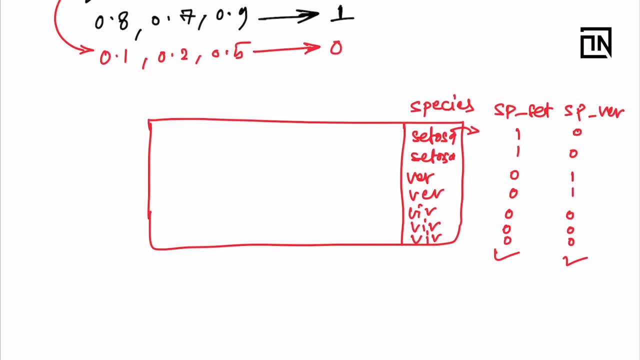 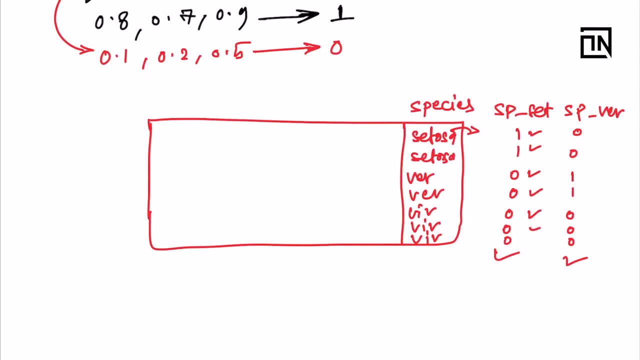 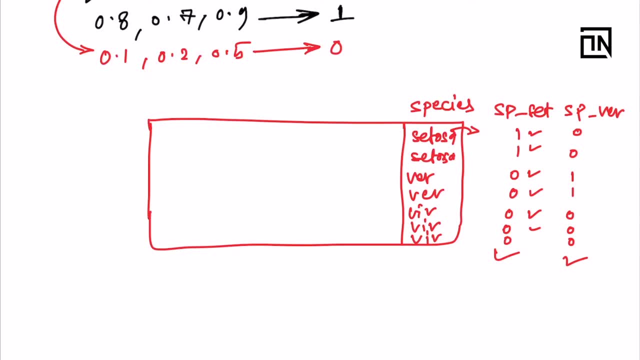 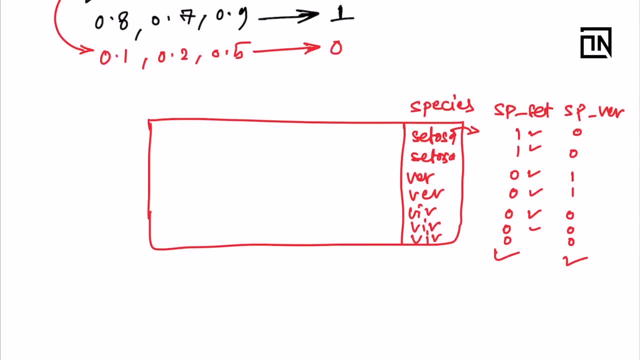 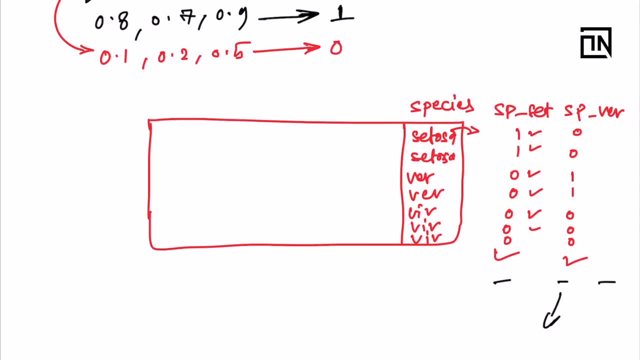 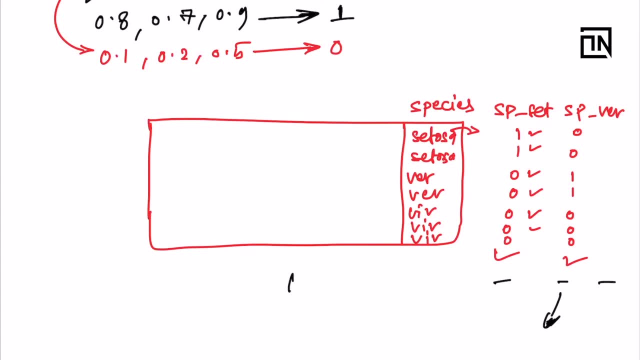 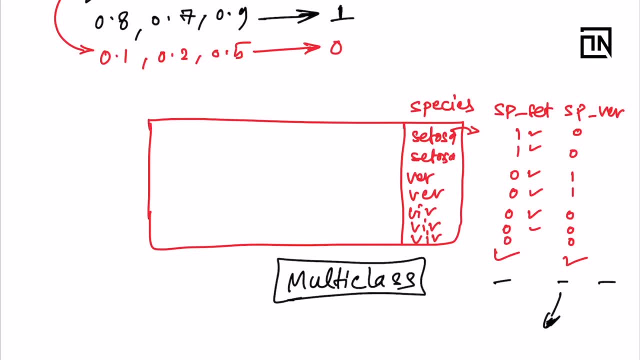 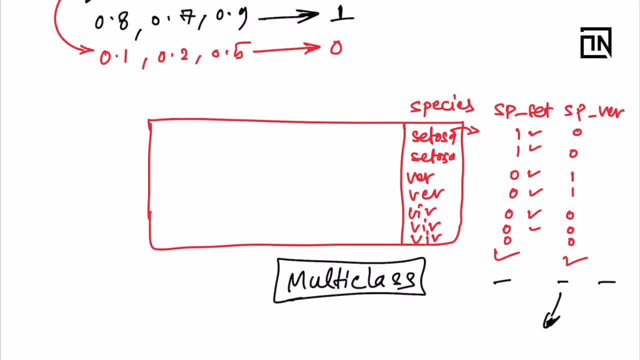 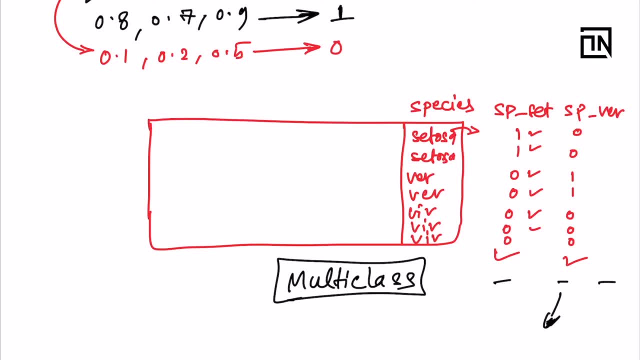 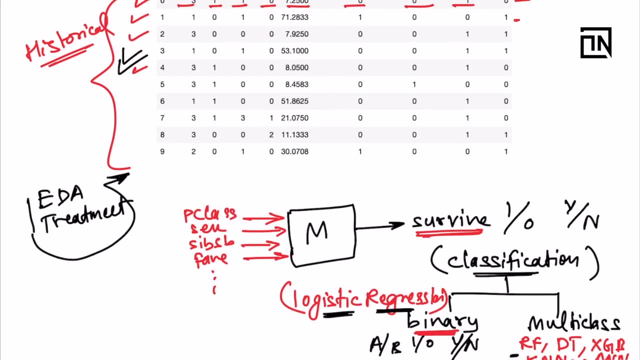 okay. so what is the set of probabilities that we are estimating and working extra hard? so, apart from this, you can use other algorithms like decision tree or random forests, etc. which are with you, okay. so this is another question, like: can't we use it or not, and what is the rational behind it? 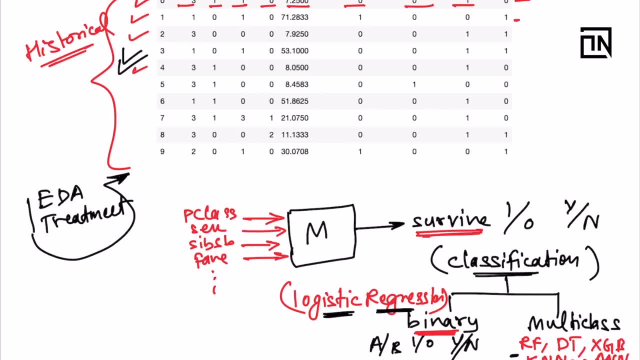 now, one more scenario where logistic regression shines is when you have huge amount of data. when there is a huge amount of data, then algorithms like linear regression or logistic regression- they work very fast and they'll be able to produce the results for you, especially like a text mining kind of. 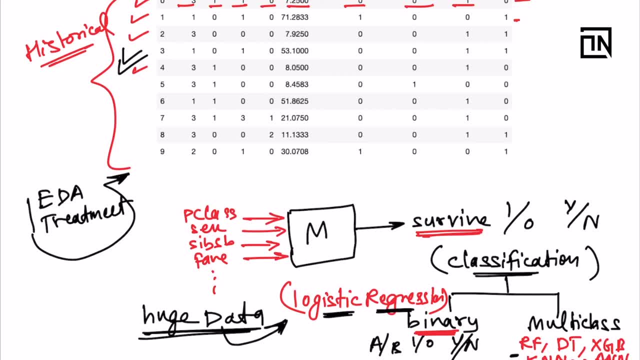 applications. or let's say you are creating applications using World2Vic or you are creating their TF IDF matrices and you are trying to do some classification based on the TF IDF scores of some text data. so they're: the cardinality will be huge, the number of columns will be really huge and the 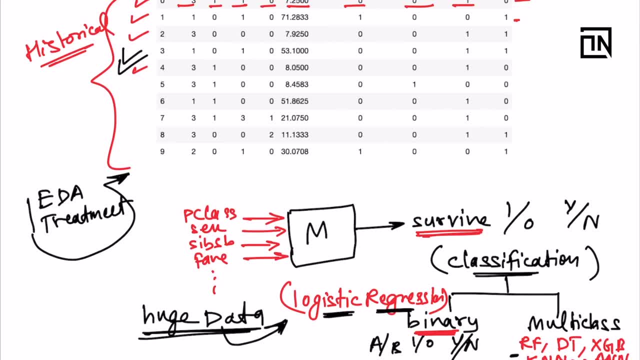 tree based algorithms will really slow down and will be painful to train, wherein the logistic regression or linear regression kind of algorithms will be very fast in these kind of high cardinality data or huge number of rows data okay. so they are very nifty, very fast. that comes in the expense of accuracy sometimes, but then if you simply don't, 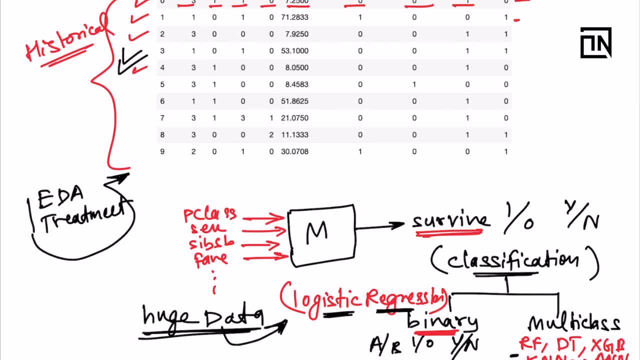 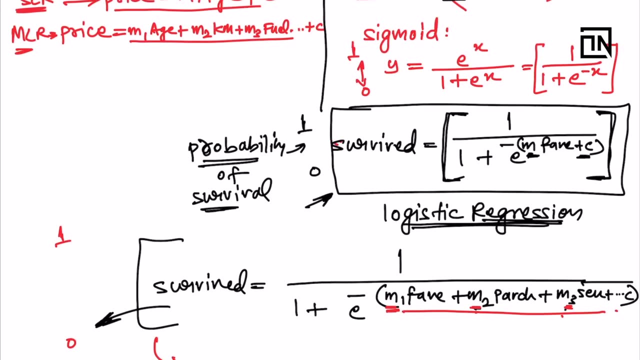 have the capacity to train the data, so at least some algorithm can come to rescue. so this is, this is another place where you can consider logistic regression, so when you are doing machine learning at scale. now i have created this equation and now i want to evaluate the results, or test my 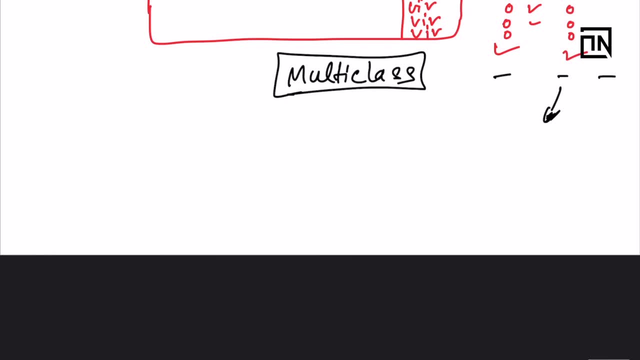 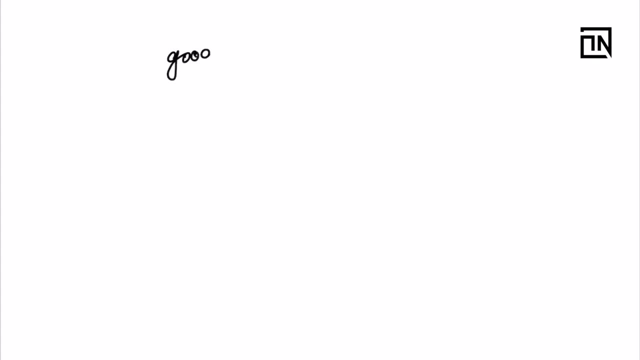 model for accuracy. so two things which you need to once again keep in mind in terms of logistic regression. first is how the goodness of fit is measured. so for goodness of fit, in logistic regression we try to use aic and bic, so any model which has the lowest value of aic or bic. 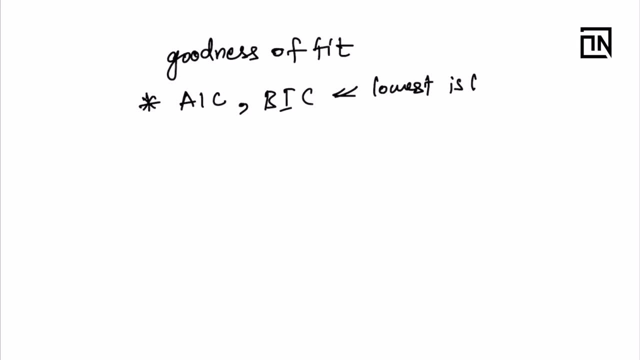 that model is my better model. now there is no standard value because it varies from data to data. so if you are using one particular data, so different set of columns will produce different set of aic and bic, so whichever set of variables or whichever set of predictors produces. 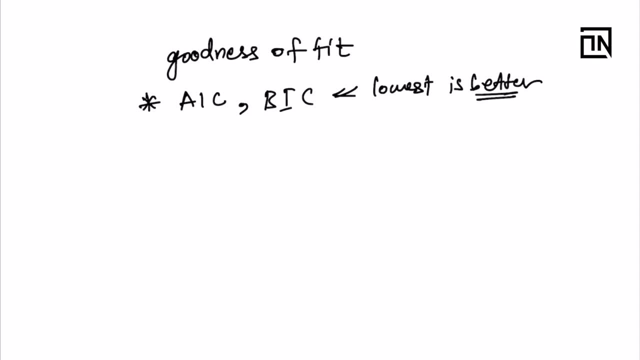 least amount of aic and bic. that must be chosen, okay. so there is a separate video for aic and bic which i have made, explaining what it is, what is the equation, etc. so try to go through that. it will help you to grasp this concept. this is also a question which is asked very frequently in the 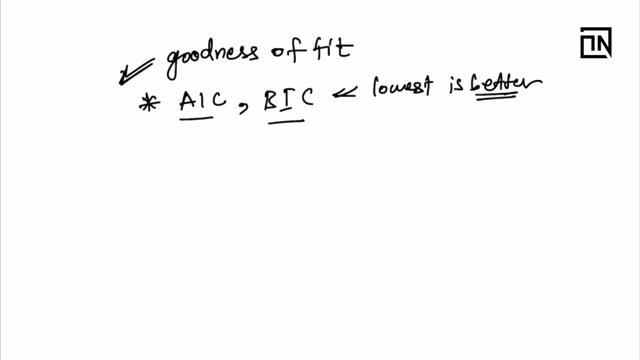 interviews. how do you measure the goodness of it for logistic regression? then, another question which is my favorite is: how did you measure the accuracy of your logistic regression, accuracy of your accuracy of your logistic regression equation? i have found this in multiple scenarios. when the candidates are answering this, they go really wrong in terms of measuring the accuracy of 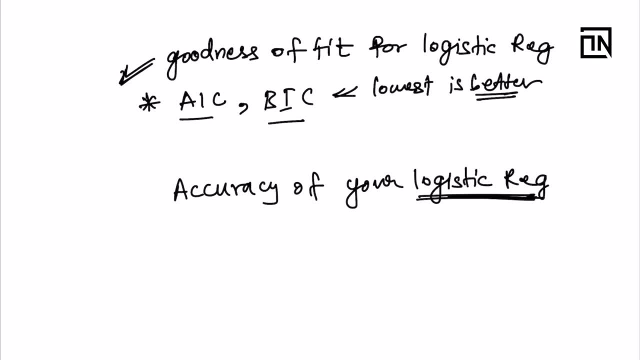 predictive models simply because they haven't done that in a real scenario. if you have done in some real scenario, you will understand the pain of explaining these terms to your clients. okay, explaining in simple terms. so the answer actually, which we use typically in the industry, is f1 score, the precision recall. 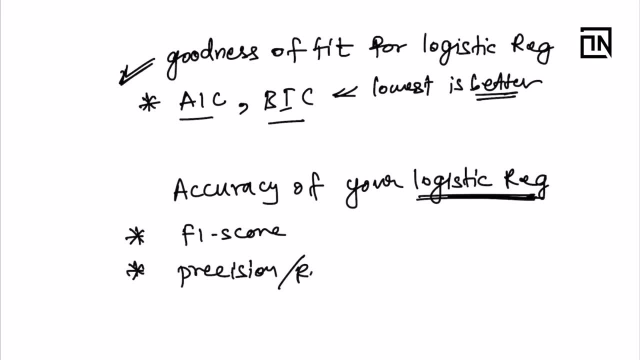 the sensitivity and specificity or the AUC ROC curve, the ROC curve and what is the area under the curve. so these are different topics or independent topics, which I have discussed in separate videos, so do check them out as well. and this is the answer for the accuracy of your logistic regression data that I measure these metrics on. 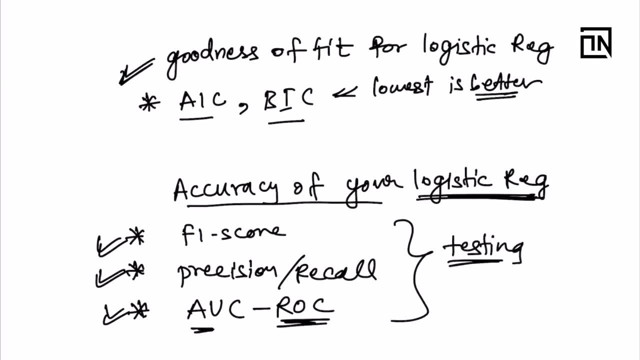 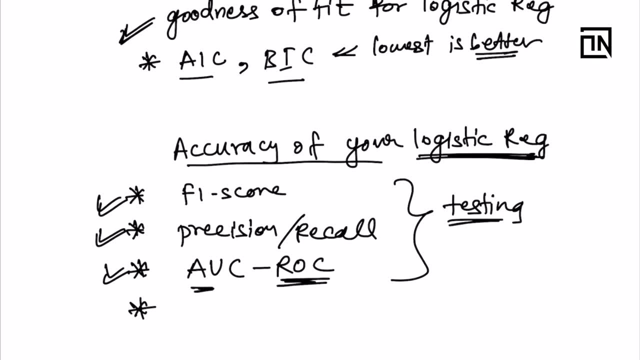 testing data and then I decide how my model is doing all right. so this is also an important question, because people confuse- oh sorry, I missed one- the confusion metrics. all of this is based on confusion metrics, so people are often confused about this. they have seen the output of the